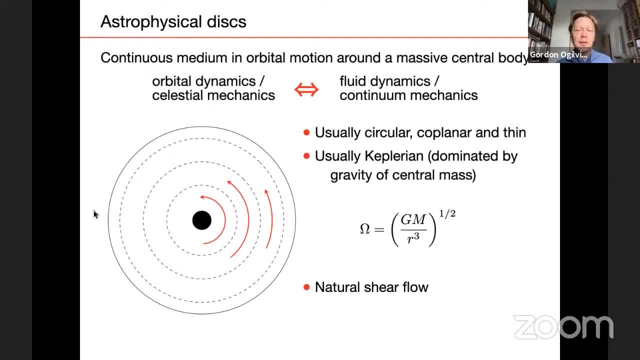 We're dealing here with material orbiting around a massive central body, a star, a black hole or maybe a planet. But the material is in the form of a continuous medium, usually a fluid, usually a gas, And there's an interesting interplay in this subject between, on the one hand, orbital dynamics or celestial mechanics and, on the other hand, fluid dynamics or more generally. 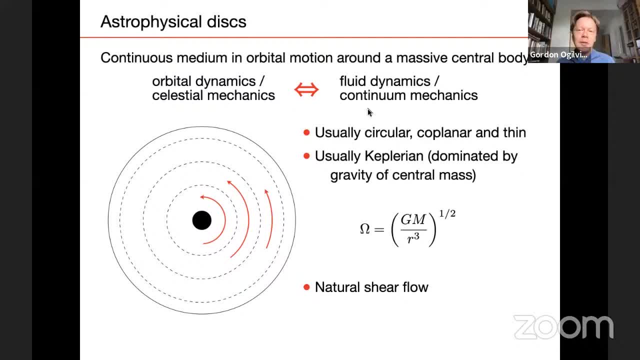 continuum mechanics. Astrophysical disks are usually assumed to be circular, coplanar and also thin, And indeed they're usually Keplerian, meaning that they're dominated by the gravity of the central object rather than that of the disk itself. So this means that the angular velocity of the circular orbital motion in a star is not the same as that of the disk itself. 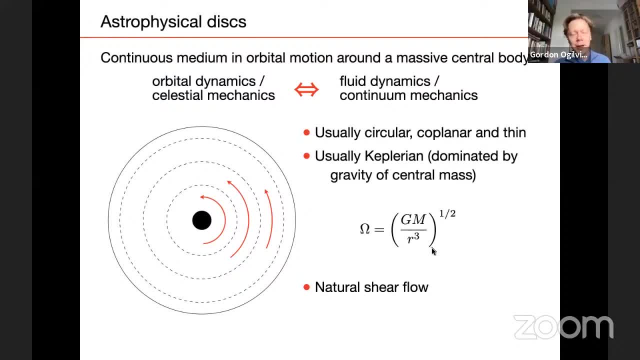 So the standard Keplerian disk is given essentially by Kepler's third law and decreases outwards in this way. So this is an example of a natural shear flow with an angular velocity that decreases outwards, and so differential rotation. Now the classical accretion disk theory is mainly concerned actually with the processes by which 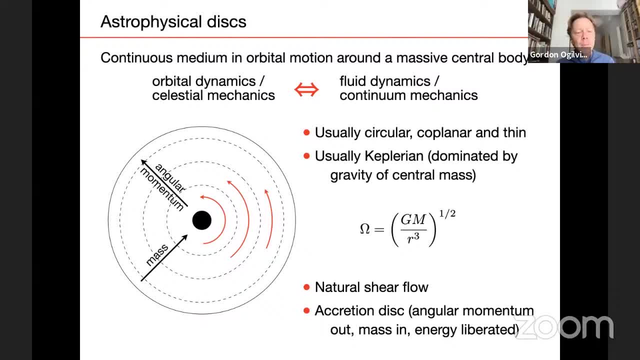 accretion disks or astrophysical disks generally evolve and become luminous and visible, and that's really all to do with angular momentum transport. So if there is any process in the disk that acts similarly to a viscosity or a frictional force, 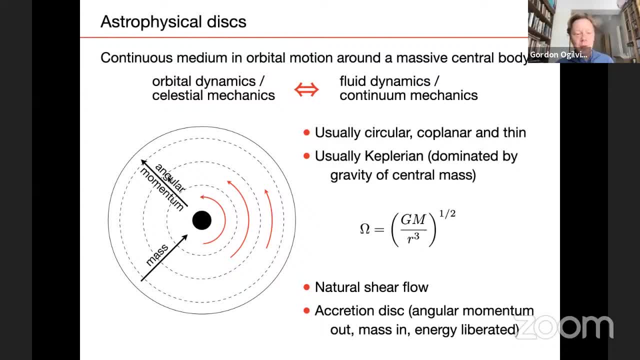 then it will transport angular momentum outwards in this shear flow, from the more rapidly rotating inner parts towards the less rapidly rotating outer parts. And if angular momentum is removed from the inner parts, then they can spiral slowly inwards towards the central object to be accreted by it. 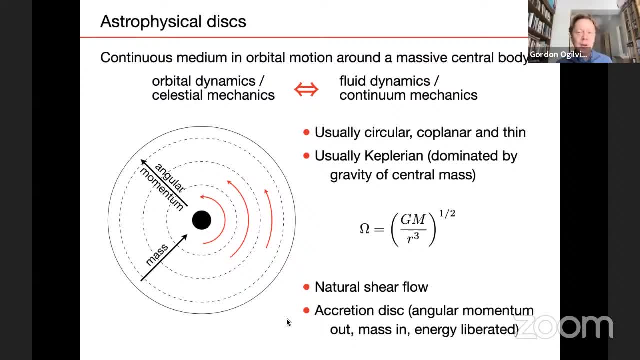 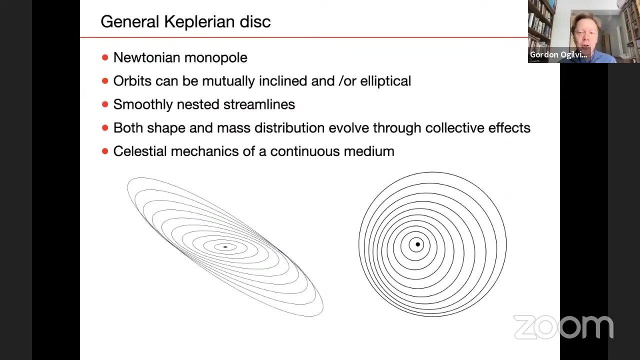 And as mass falls into the gravitational potential, well, it liberates energy, making the disk hot and luminous, and indeed some of the most luminous objects in the universe, Such as active galaxies and quasars, are powered by this mechanism. Okay now, I've been interested for quite a while in a more general concept of a Keplerian disk. 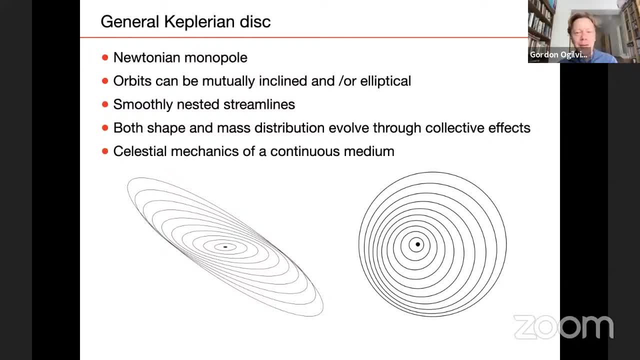 and we know that around a Newtonian point mass, the orbits can generally be inclined at any angle or they can be elliptical. And you can consider a Keplerian disk made up of these variably inclined or variably elliptical orbits. And I mean to the extent that the motion of the material in these thin disks is dominated by gravitational and inertial forces. 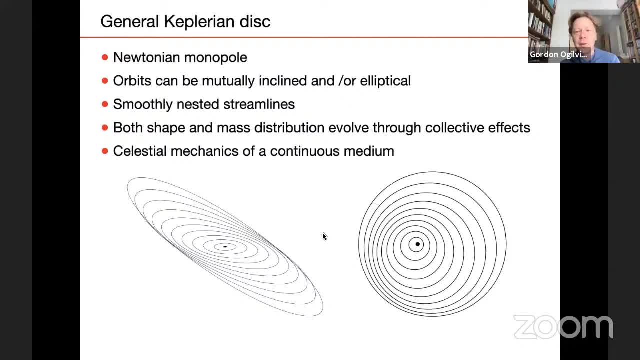 these orbits can be seen as the first approximations to the streamlines of the, the gas flow in the luminous Kepler, these disks. So it's very important that these orbits are closed and they don't intersect their neighbors. At least that's true if the eccentricity varies sufficiently slowly with. 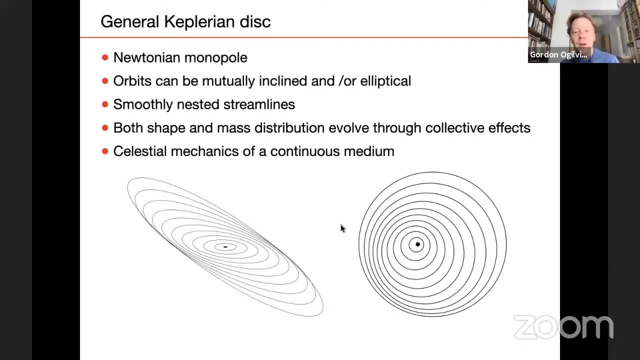 the size of the orbit. So then we can imagine these as gas streamlines that are not in conflict with each other. They don't produce any shocks or anything like that. But having set up a disk of this form, it's then appropriate to ask: well, not just the mass distribution, but also the shape. 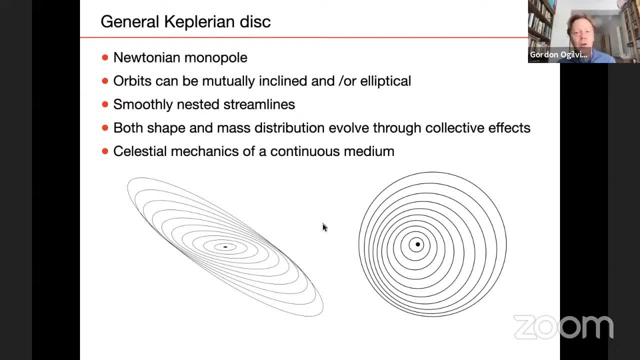 of the disk. How do they evolve on timescales long compared to that of the orbital motion as a result of the various collective effects in the fluid. So that might include what's called viscosity and accretion disk theory, which is usually really a label for turbulence and turbulent. motion. So that might include what's called viscosity and accretion disk theory, which is usually really a label for turbulence and turbulent motion. So that might include what's called viscosity and accretion disk theory, which is usually really a label for turbulence and turbulent. 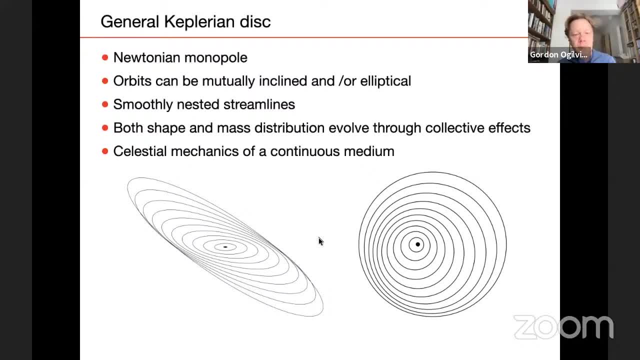 stresses or possibly wave processes, But actually just the pressure in the disk and its self-gravity. they contribute to the communication of, or the evolution of the shape of the disk, as we'll see Now. in some sense this can be thought of as the celestial mechanics of a 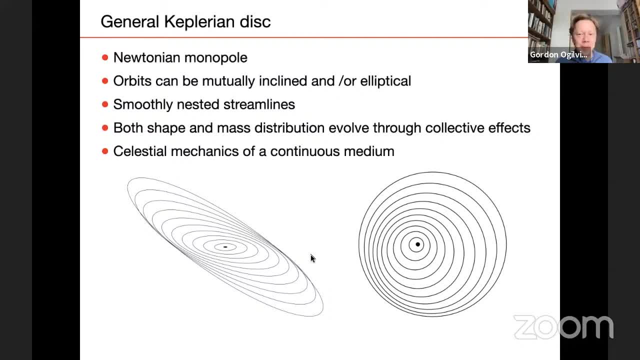 disk. Basically, Keplerian orbits evolve or are perturbed by various other perturbing forces which might come from, let's say, other planets in a multi-planet system, like the solar system, or whatever other forces other than that of the central body act on particles or minor bodies. 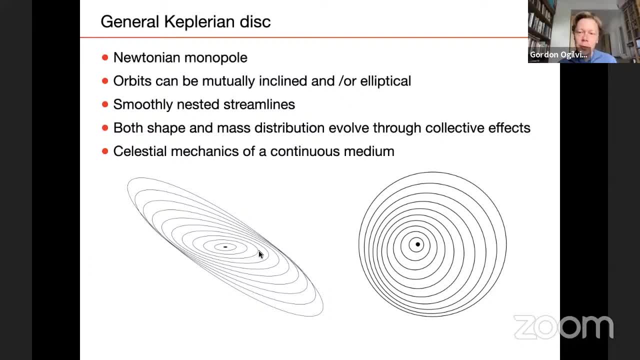 Now for these fluid disks. there are various forces that are involved in the distribution of the disk. There are forces that are causing perturbations from the basic orbital motion, And some of those forces are internal to the disk. They arise from the stresses in the fluid, which might just be. 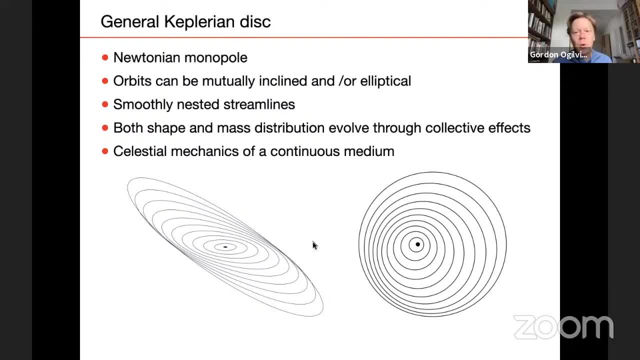 pressure, but they could also be turbulent stresses or magnetic fields. There can also be external forces due to companion objects and so on. Okay, well, we're actually hosting a workshop next week in Cambridge, or virtual workshop, which is entitled The Dynamics of Distorted Disks. 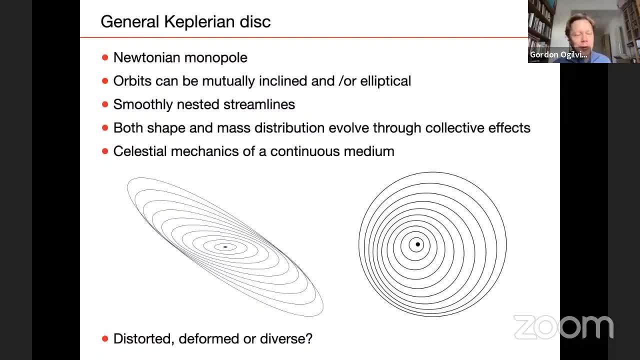 And I mean these have sometimes been called distorted or deformed, but perhaps we should just think of these as more diverse and think about the diversity of Keplerian disks that are possible in nature. So I mean, do these actually occur? Certainly there's a lot of evidence and a lot of theoretical reasoning as well, for considering warped and eccentric disks. A disk can be expected to be warped basically whenever there's a misalignment between the original plane of the disk and almost anything else in the system. 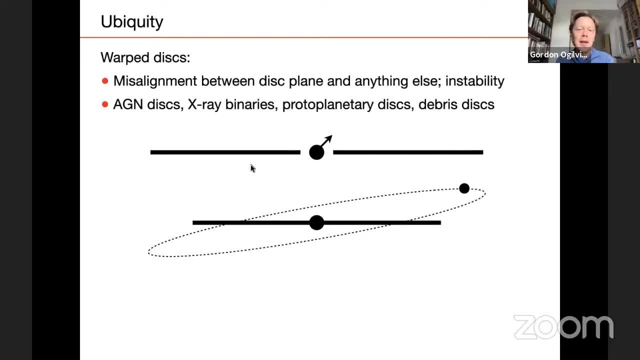 So a classic problem investigated since the 1970s, is where a disk has formed in a certain plane, plane around a black hole, but the spin axis of the black hole is not perpendicular to the disc plane, So I mean the plane. the original plane of the disc will be dictated by the 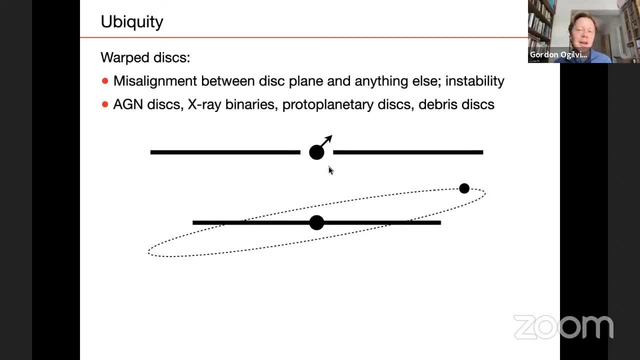 angular momentum vector of the material that forms the disc and that may be unrelated to the spin of the black hole at the center. So here we have material orbiting not in the equatorial plane of the black hole, so it'll be subject to gravitomagnetic torques, leading to 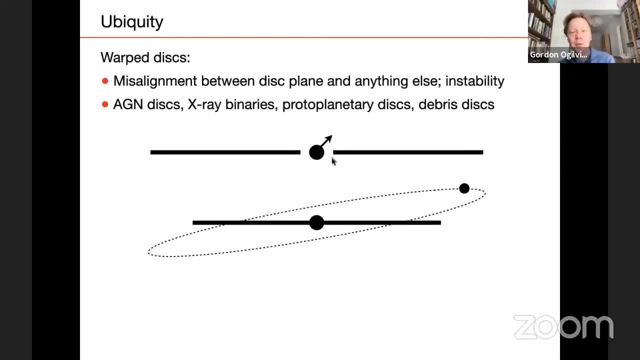 lens-attiring precession, which will vary strongly with the radial size of the orbit, and that tends to cause a twist and a warp in the disc. So a classic problem is to try to work out the steady shape of the disc in this situation. But other sort of misalignments might include. if we have an orbital companion, like a binary star or a planet with an inclined orbit- inclined with respect to the original plane of the disc- then the disc will become non-planar as a result. As for eccentric discs, well again. 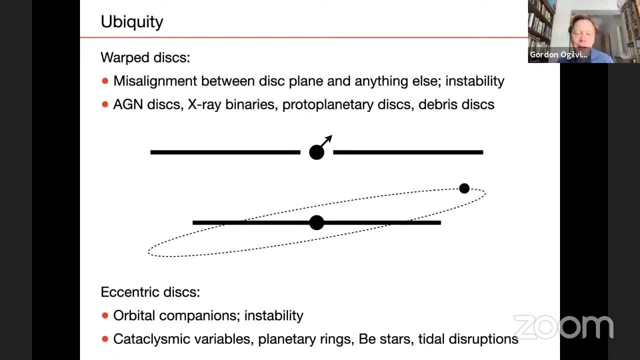 eccentricity can be induced by an orbital companion. Actually, even if the companion has a circular orbit, well, if the companion has an elliptical orbit, then it's unaligned. So if the companion has an elliptical orbit, then it's unaligned. 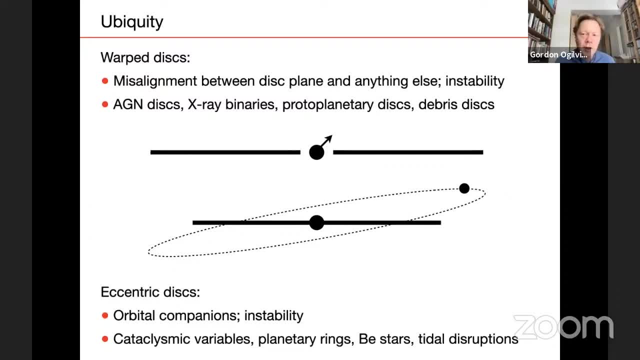 Basically through secular forcing of the disc it will acquire some eccentricity. But even if the companion has a circular orbit, then there can be mean motion resonances that lead to an instability that produces eccentricity in the disc. I'll show examples of that. 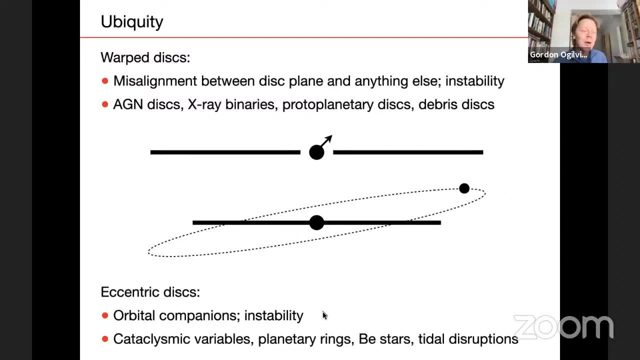 And from the observational point of view, there's good evidence for eccentric discs in interacting binary stars, such as the cataclysmic variable and the, the tidal disruption events where stars are torn apart around black holes in galactic nuclei, producing highly elliptical. 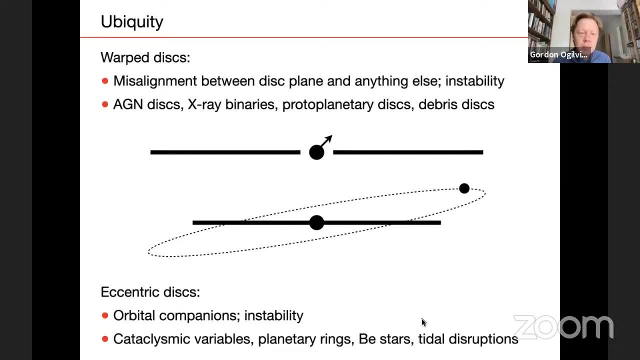 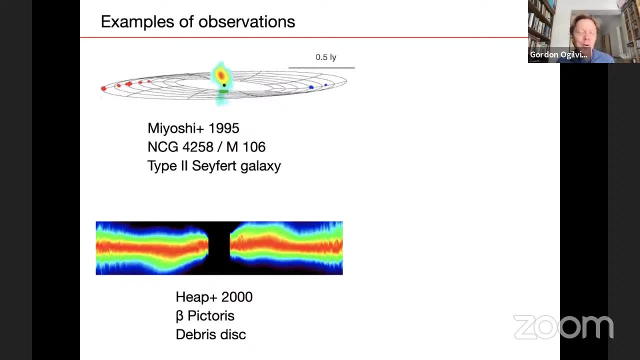 accretion discs. There are relatively few direct observations of the actual warps or eccentricity, but here are some examples. Maser emission from this active galaxy, and a few others, has enabled us to trace out the shapes of warp discs in these galactic nuclei. 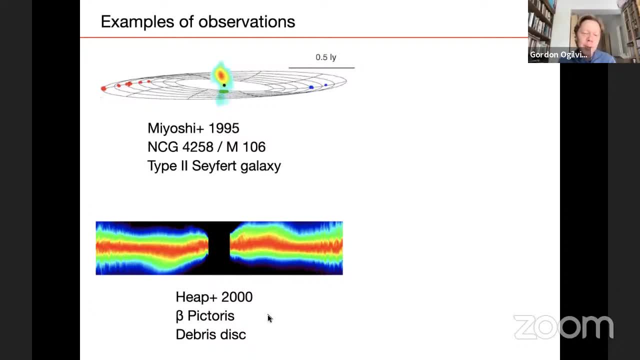 And this is a well-known debris disc around the young star Beta Pictoris, where there's a warp which is thought to be associated with planets. I'd like you to take a closer look at also several other cases where walk variants are associated with ancient planet- learnt noir damage. 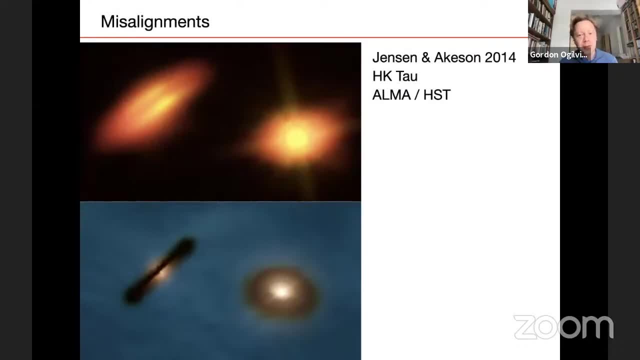 There are more observations of misalignments from which we would deduce that warps are likely to occur. so here's a young binary system with both models that combine your Alma disc and steps to be aggregated. Here is that young binary system. this is the observations from Alma and Es쓴. invasion ACT. 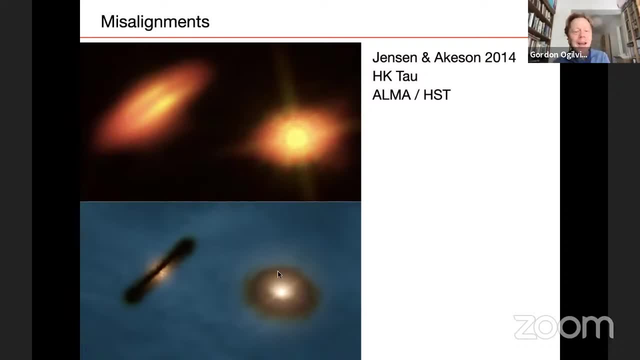 in May, befitting of the Ф. President of the information galaxy. it's used for paisage thanks to its many- Brettonanne's mission, ALMA and HST, and this is the artist's impression of the system. The point is that each of these 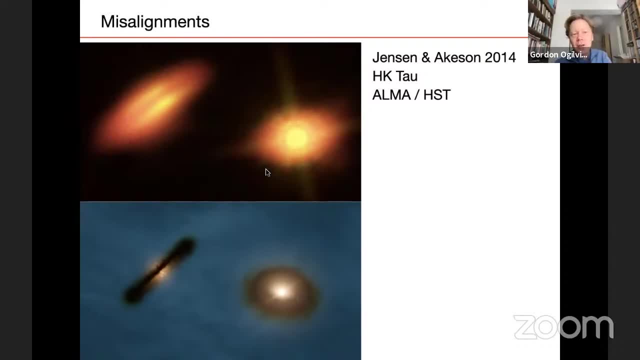 two young stars has a disk around it, and each disk is measurably misaligned with the plane of the binary orbit. So we should expect each of the disks to be warped at some level, although that can't yet be measured directly. Another type of observation that's been prominent recently: 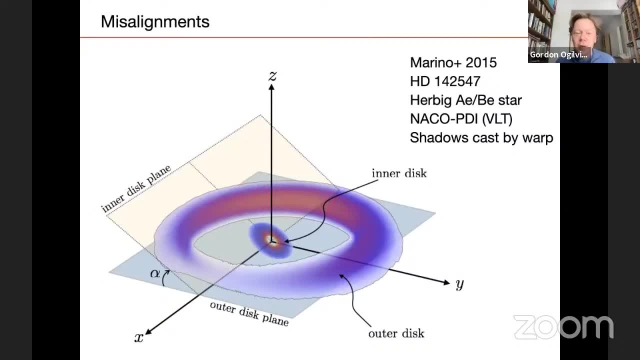 is well, there's been a lot of developments of imaging of disks around young stars, and here's an example of where shadows in the outer parts of the disk, which move quite rapidly, have been interpreted as being cast by a strongly misaligned inner part of the disk that's processing and casting. 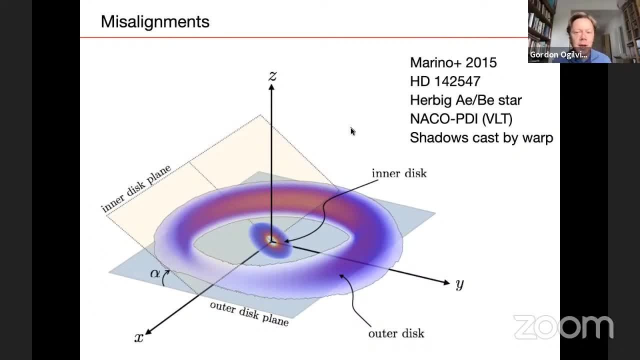 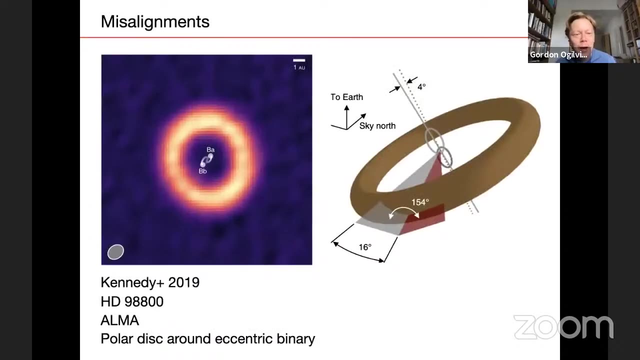 a moving shadow on the outer part of the disk. So there are several systems like this where strong misalignments have been deduced and associated with warps. Here's a very extreme example of a misalignment where, well, we have a highly eccentric binary. 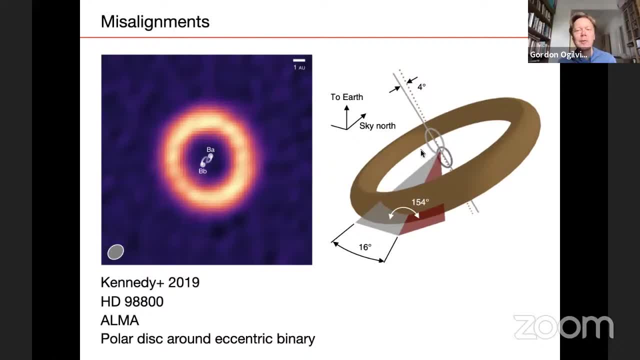 star And a disk, well, in the form of a ring, has been found around this eccentric binary, and the disk is basically perpendicular to the plane of the binary orbit. It's in a so-called polar orbit, and there is some nice theory about how the disk finds its way into this polar alignment. 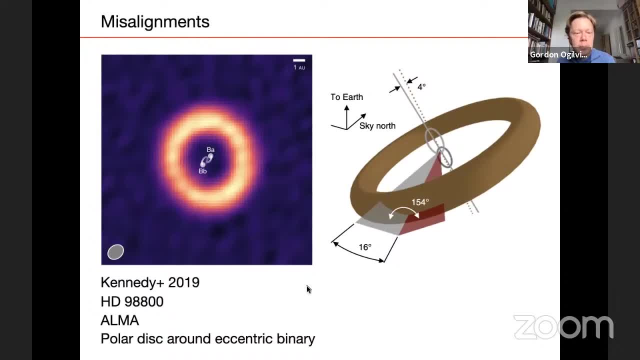 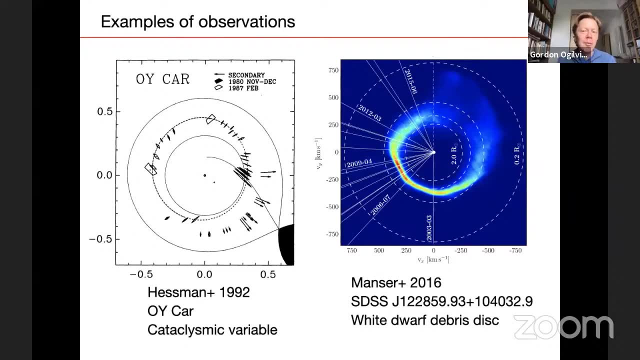 because of the eccentricity of the binary orbit. As for measurements of eccentricity, well, there are a lot of these. in disks There are relatively few, but here's an old example. This is one of these cataclysmic variable interacting binary stars of the super hump category. 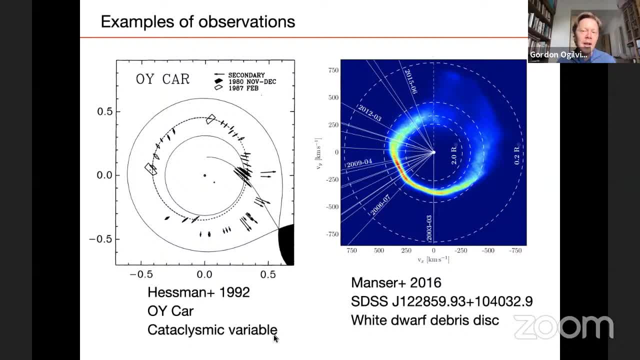 where, during a so-called super outburst, the accretion disk becomes elliptical and starts processing, And in this case, through the eclipse mapping technique, they were able to map out the elliptical shape of the rim of the disk. Now, more recently, this is an observation of a debris disk around a white dwarf, where some 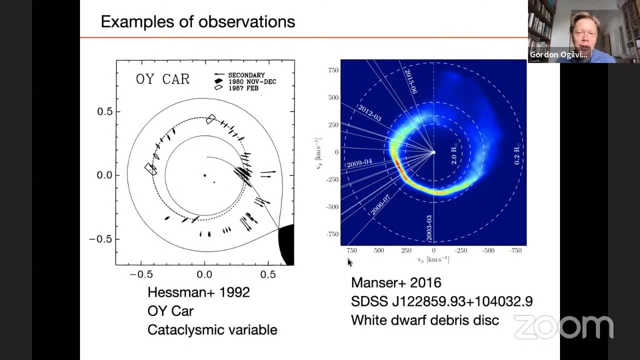 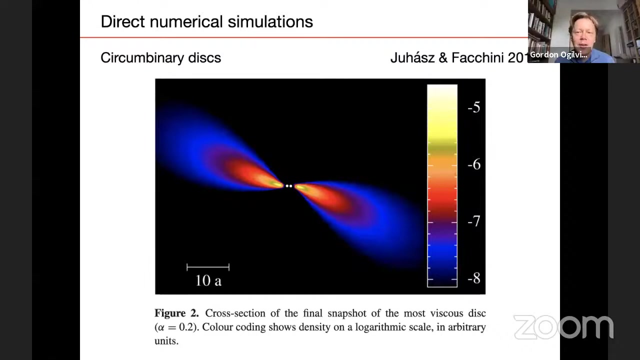 material of planetary origin is being disrupted, producing a debris stream and an elliptical disk that's processing, And there are several systems where this procession has been detected. OK, Now, there's been a good amount of work using numerical simulations, much of it using the SPH method. 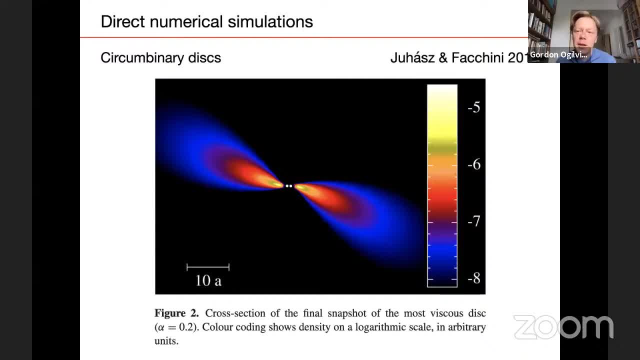 So here, for example, is a simulation using the SPH method of a tilted disc around a binary star or binary system. So the disc is initially tilted at some angle with respect to the plane of the binary orbit. so the country of application is highlighted here. 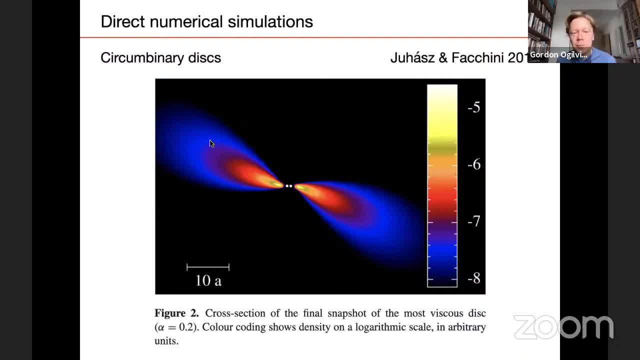 And then it's now tilted slightly to the right. that's juicy but not totally sensational. but it's speed riveted orbit And in this case it develops a smooth warp connecting the orientation at large distance and then it lines up with the binary orbit at smaller radius. But what's been found in this? 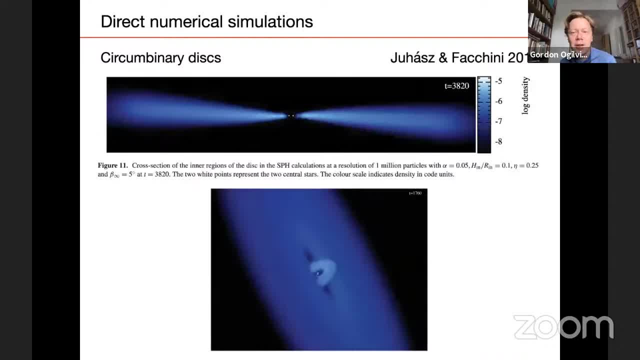 type of calculation is that in certain regions of the parameter space, particularly if the disk is sufficiently thin and not so viscous, and if the tilts are large, then there's a tendency for the disk to break into distinct segments. So, rather than having a smooth transition, a smooth warp. 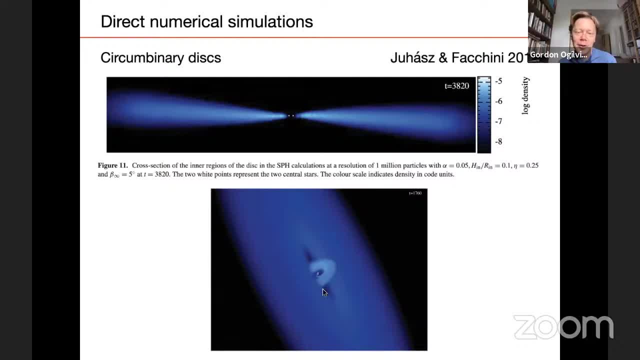 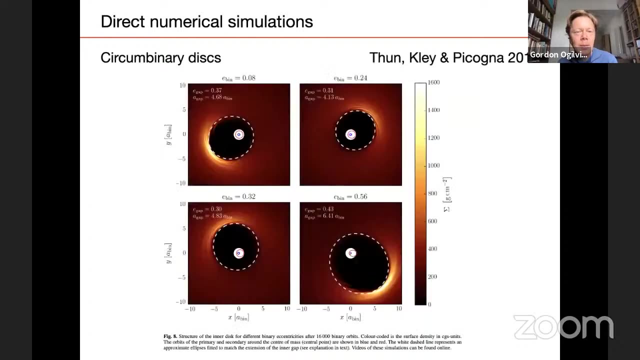 rather, the inner part of the disk breaks off and has only a very tenuous connection with the rest of the disk, And that allows it to process essentially independently of the rest of the disk. So that's one of the interesting phenomena that's been revealed. Now these circumbinary disks have also been studied quite a lot in basically a 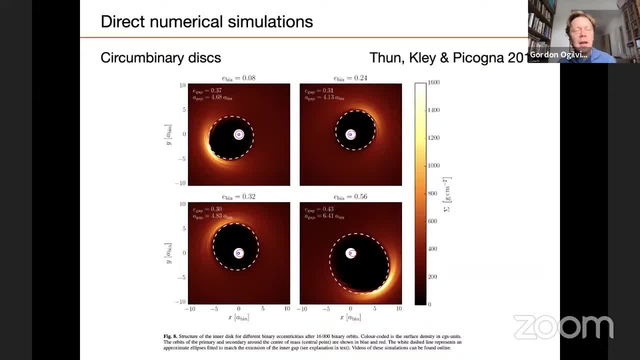 two-dimensional configuration, without or without any tilt involved, And there it's found that they typically become eccentric, even if the central binary, in fact especially if the central binary- is circular. So initially this case eccentricity can develop in the disk as a result of a resonant interaction between the 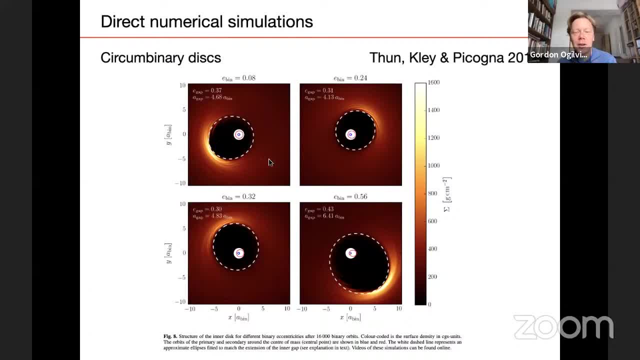 motion of the binary and the motion of the surrounding disk, leading to a growth of eccentricity, And that we see this elliptical cavity then, which processes around and that causes a whole lot of interesting phenomena, including modulation of the accretion rate onto. 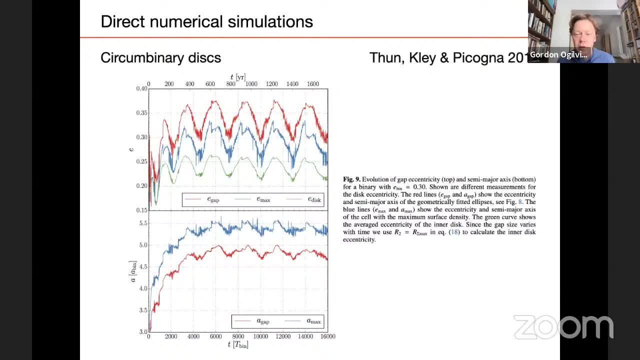 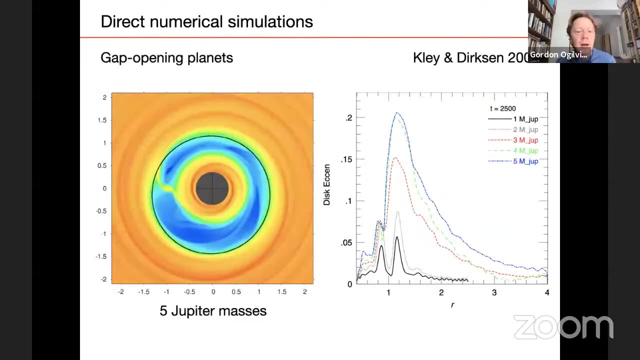 the system and can have important consequences for the evolution of the binary orbit. So this is important for both young stellar systems and also binary black holes. Okay, well, related phenomena are also seen in the planet-disk interaction problem, So here is a. 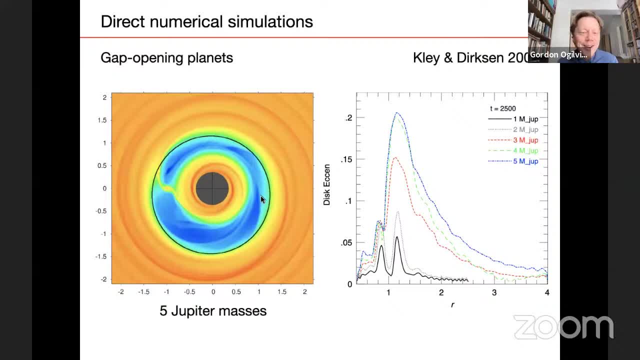 simulation by Willy and his robot- One of his PhD students some years ago, of planet-disk. so there's a planet of five Jupiter masses on a fixed circular orbit and it opens a deep gap in the disk. But at least for these, 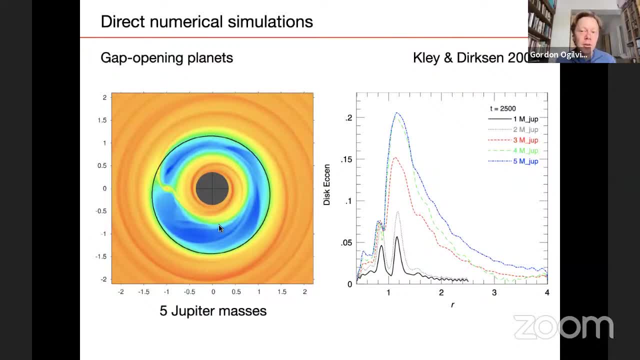 parameters. the disk is found to become eccentric through this. well, through a mean motion, resonant interaction, essentially leading to eccentricity, particularly in the disk exterior to the planet's orbit. So that can affect things like the accretion of mass onto the planet, so it affecting its growth, it can affect the 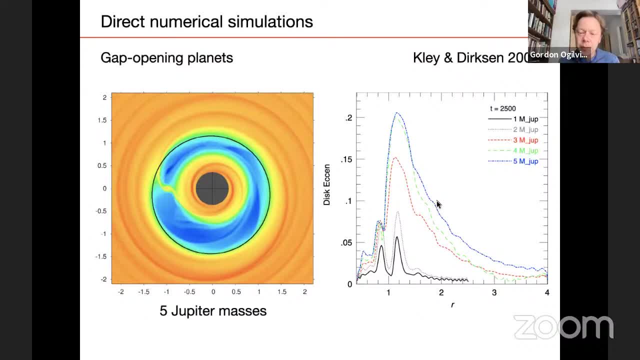 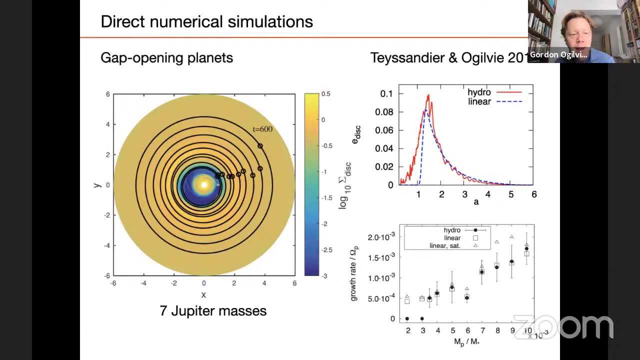 migration of the planet and so on. Yes, we attempted to explain the growth of eccentricity in this type of system through a linear theory, basically explaining how a certain eccentric mode in the disk acquired a positive growth rate through various mean motion resonances. 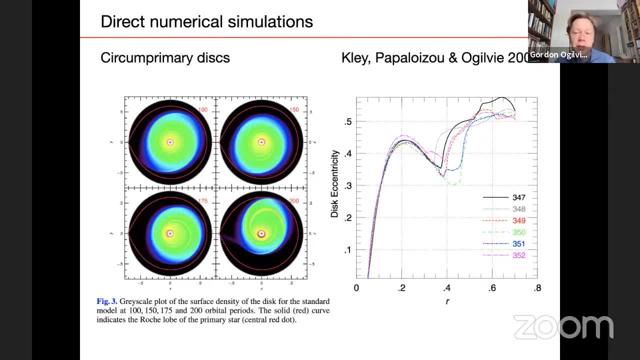 Okay, well, and all this ties in in some sense with the super hump phenomenon in those interacting binary systems where there's a particular mean motion resonance that's thought to cause eccentricity in the disk, And for many years that was only found in SBH simulations. 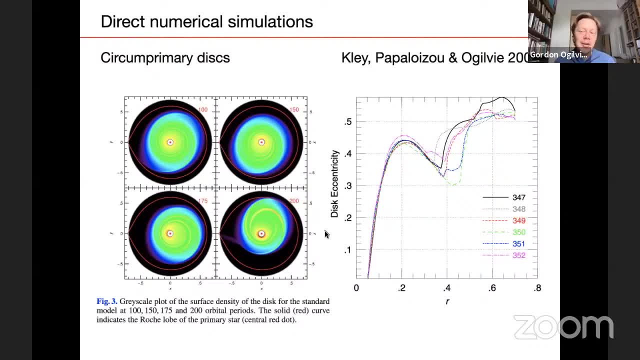 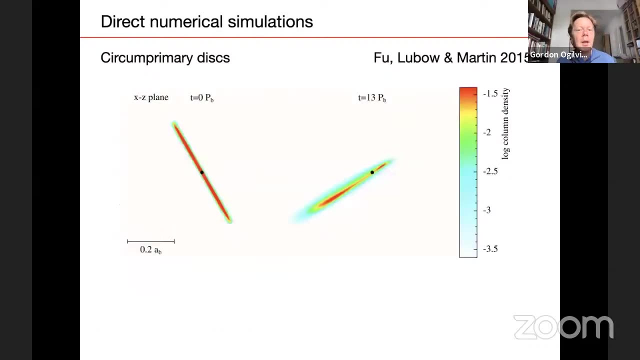 Grid-based simulations didn't produce this- any eccentric disks, But well again, with Willy a number of years ago we were able to see this phenomenon occur in a grid-based simulation for the first time. Another interesting recent development has been what involves a combination: 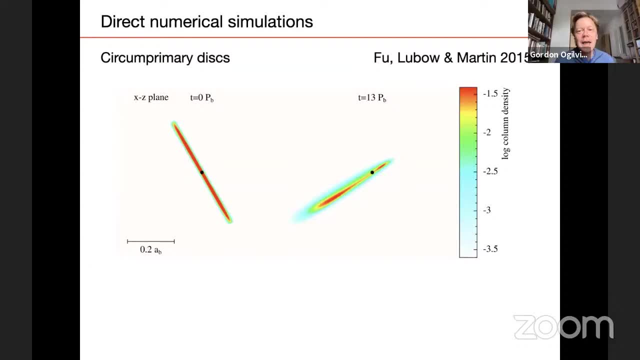 of warping, or at least tilting and eccentricity. So this is SBH simulations of disk around a star in a binary system. And here the disk is initially tilted at a large angle with respect to the binary plane, So larger than well larger than 40 degrees, we'll see. 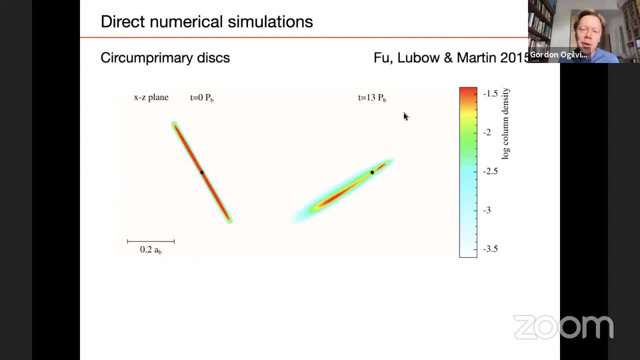 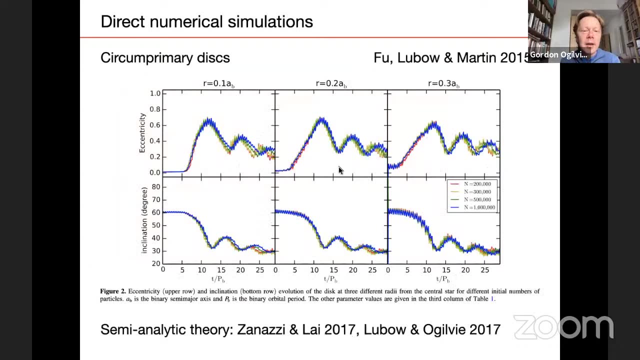 is important Because after a number of binary orbits the disk becomes highly elliptical And this is how the eccentricity varies in time in this type of simulation. So there's a large growth of eccentricity and then damped oscillations because the disk in this simulation 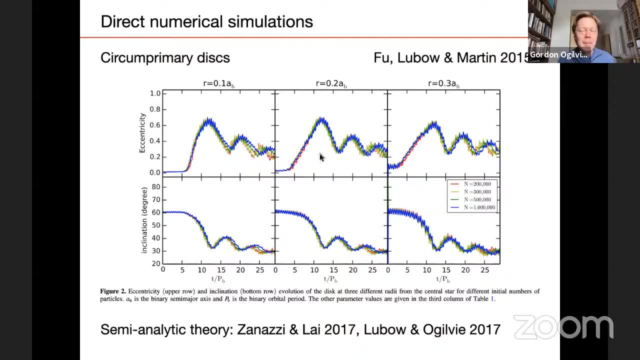 is highly dissipative and it damps out the eccentric mode that results. So this can be understood as a continuous analog for a disk, rather than a particle of the Lidov–Kozai process that's quite well known in celestial mechanics. 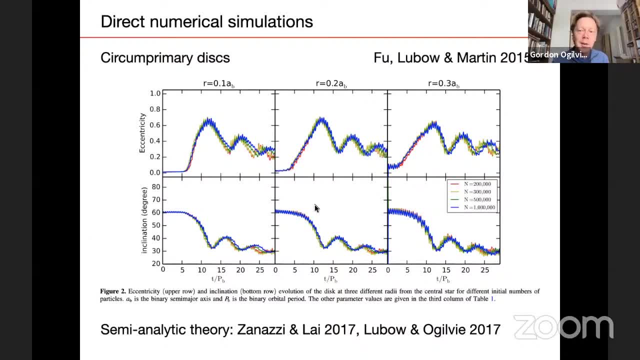 whereby an orbit that's sufficiently inclined by more than about 40 degrees with respect to the orbit of an outer- let's say, binary- companion, becomes highly elliptical and there's an oscillatory exchange between inclination and eccentricity in this system. So we can see that this is a very, very similar process, but it's also a very different kind of. 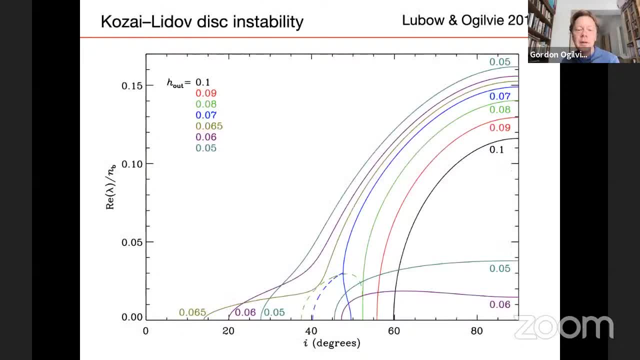 oscillatory exchange between inclination and eccentricity in this system. So we can see that this is a highly elliptical process and there's a very large growth of. We helped to develop some semi-analytic theory of this, in which a disk that's tilted through. 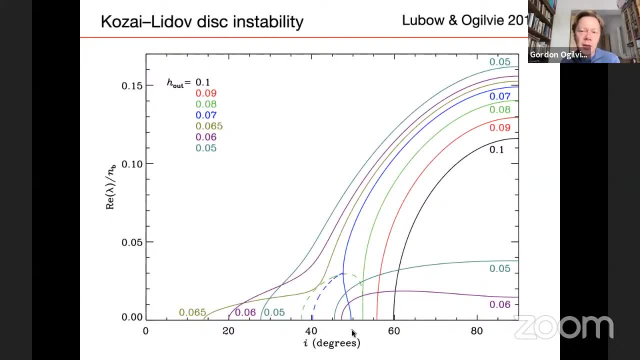 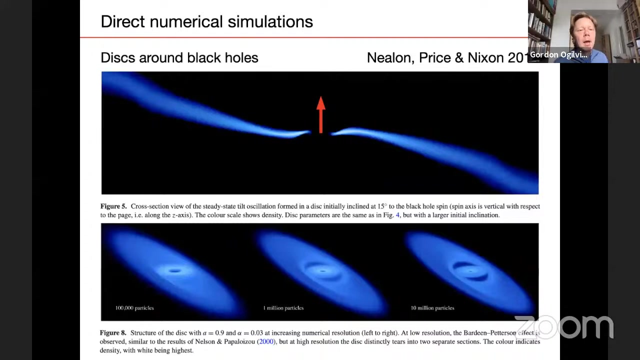 a sufficiently large angle develops an unstable mode. This is an initially circular disk. The eccentric modes in the disk become unstable through this Lidov-Kozai process and growth rates can be obtained depending on the parameters of the disk. There's also a lot of interest in disks around black holes and simulations of this process. 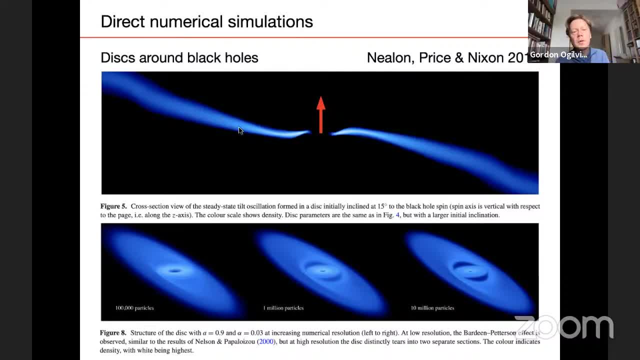 in some cases produce smooth warps, although here's an interesting example of where, contrary to the classic Bardeen-Peterson effect, the variation of the tilt angle with radius is non-monotonic. We see the beginnings here of an oscillation. 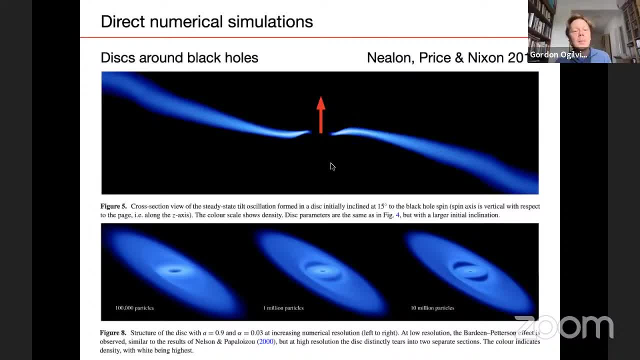 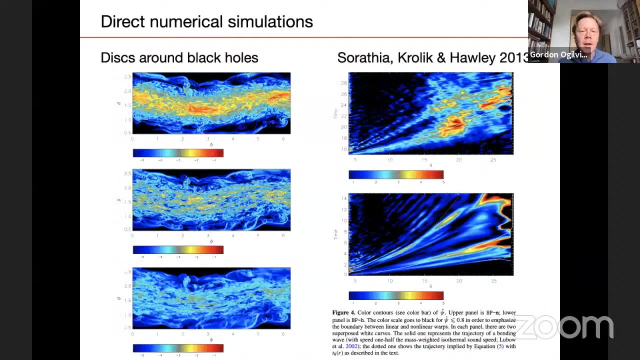 Which was predicted theoretically. But again, if the tilts are sufficiently large or the disk is not very thick or viscous, then there's a tendency for the disk to break into independently processing segments like this. Okay, now some researchers have been able to do this type of simulation with. 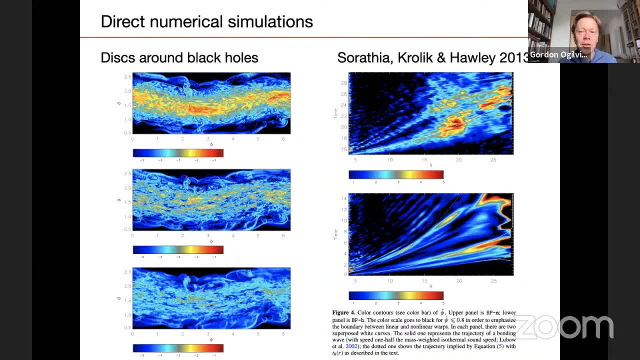 sufficient resolution and with grid-based methods to capture the MHD turbulence in the disk resulting from the magnetorotational instabilities. These are very challenging computations, and perhaps some other things have been compromised to make this possible. Most of the simulations that I showed before are just treating the disk as a viscous. 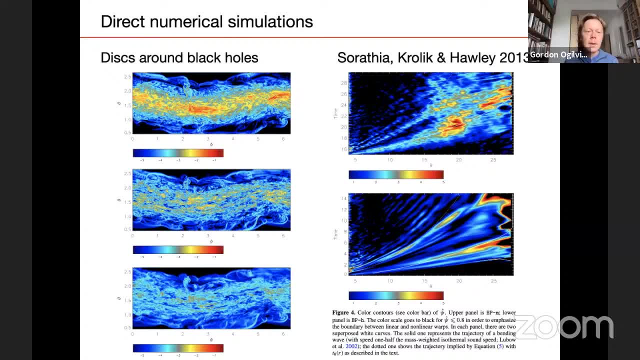 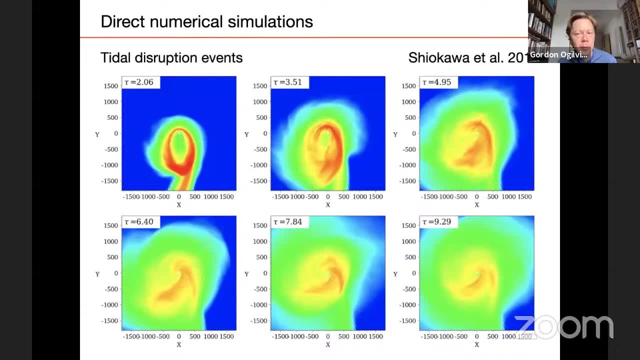 laminar flow. Okay, I should also briefly mention tidal disruption events, because, at least in some of the simulations of tidal disruptions, where a star encounters the black hole at the center of a galaxy on a highly elliptical or parabolic orbit, what's produced is a highly 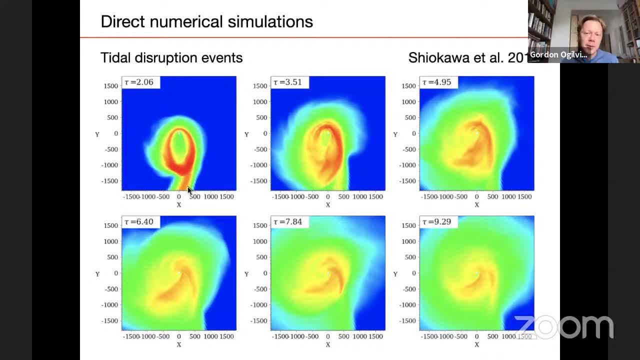 elliptical accretion disk, Although in some other simulations, depending on the thermal physics involved, there can be a lot of circularization before the accretion occurs. But this is certainly an important situation that we've been investigating to understand the dynamics of the 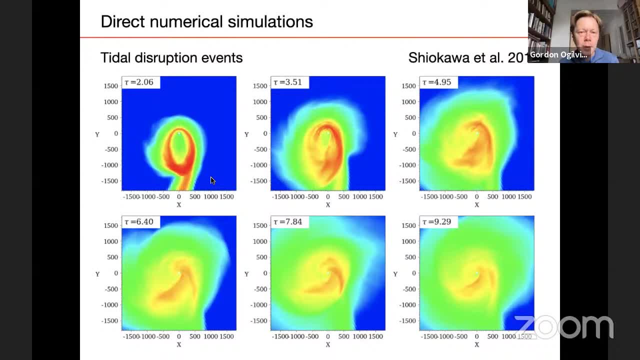 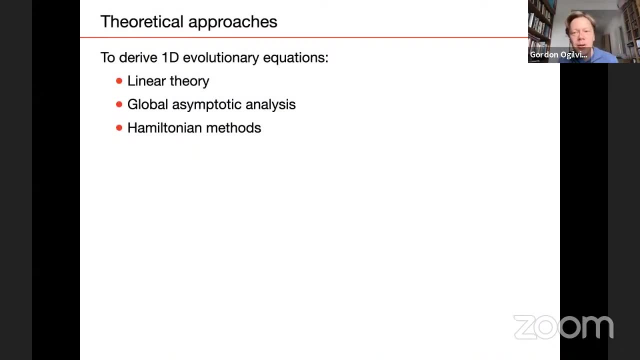 elliptical accretion disks in this type of situation. Okay, well, what can we do in terms of theoretical approaches other than global numerical simulations? here There's quite a long thread of work attempting to derive essentially one-dimensional evolutionary equations describing how these systems behave. One approach is to use linear. 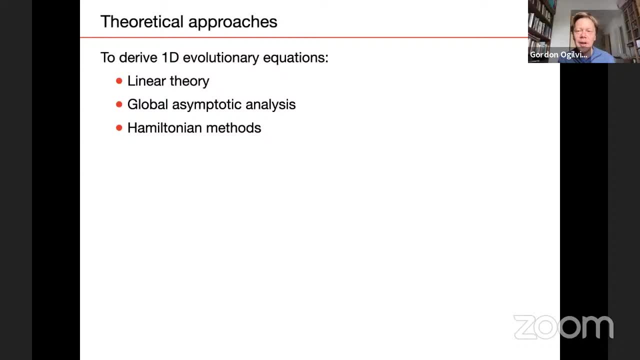 theory. So you regard the eccentricity or the inclination as small perturbations of a standard circular coplanar disk and then you can develop some linear theory describing how the eccentricity and inclination evolve, which may involve growth or decay and wave-like propagation. 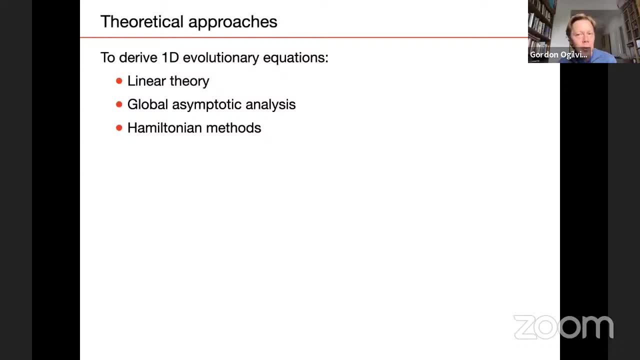 When they're not small. we need a more non-linear method and I've been involved in some global asymptotic analyses where we're basically making use of the fact that the disk is thin and that there are separations of length and time scales in the problem to derive evolutionary equations. 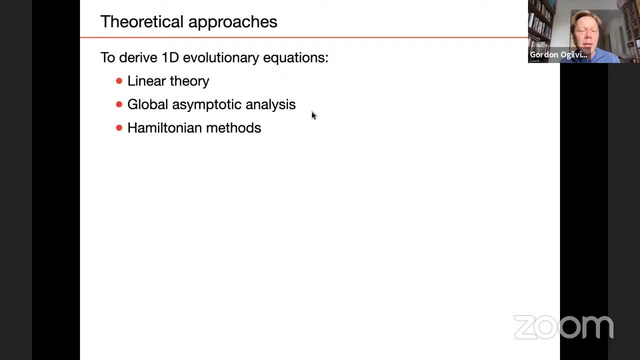 through asymptotic methods, And I'll say a bit about that in a moment. More recently, I've also been trying to use variational methods to derive these equations, and I probably won't say a great deal about that here, but it does provide. 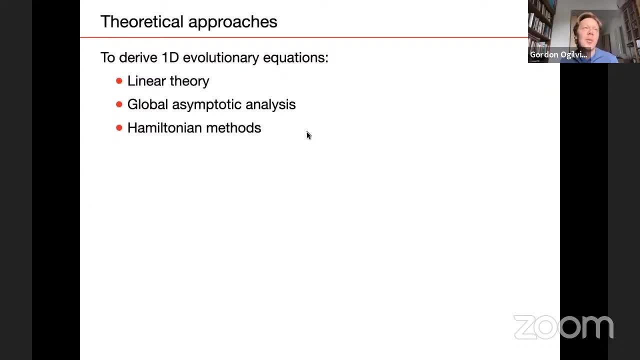 I think, some useful insight into what is otherwise a rather complicated set of equations. Another approach that I've been developing is to derive some reduced computational models, alternatives to the global numerical simulation. I'm interested in what can be done using local computational models to study these. 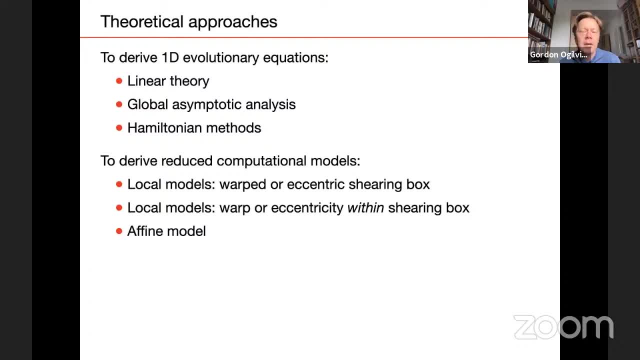 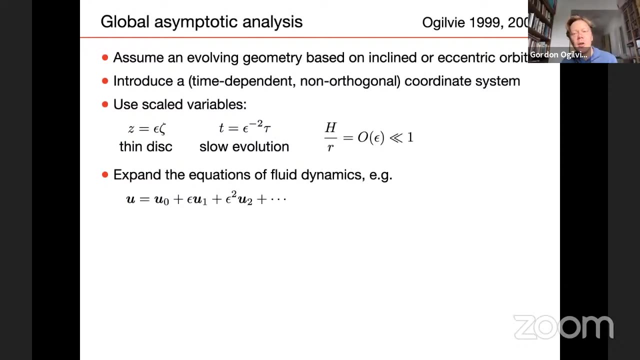 the physics of these situations, And I'll also say a bit about an affine model that I developed to reduce the problem basically to a two-dimensional one. Okay, so the global asymptotic methods that I developed. roughly speaking, it goes like this: 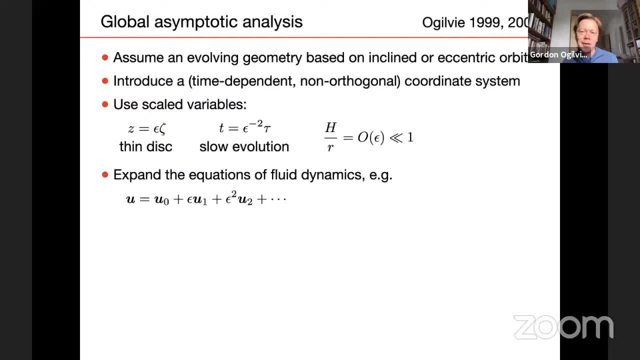 You assume that you've got either a warped or eccentric disk which has some geometry that is slowly evolving and it's based on the geometry of a family of Keplerian orbits, And then we introduce a coordinate system that's adapted to those orbits. 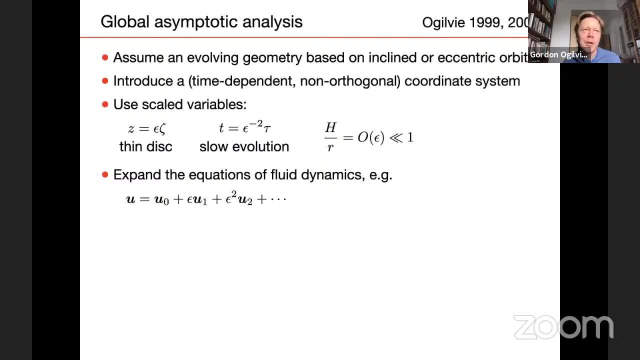 It is somewhat complicated because it's a non-orthogonal coordinate system. It's also time-dependent, although only slowly. It evolves on a time scale much longer than the orbital time scale. But basically this is using a classic asymptotic technique. The disk is thin. 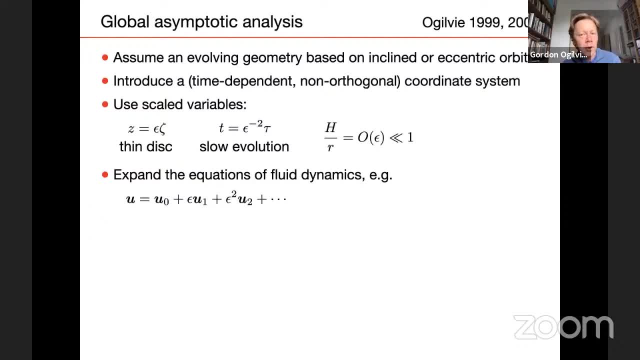 so we introduce scaled coordinates to resolve the internal structure of the disk and to capture its evolution on time scale much longer than the orbital. And then the equations of fluid dynamics are expanded in powers of a small parameter, which is essentially the aspect ratio of the disk, which is also a measure of the sound speed relative. 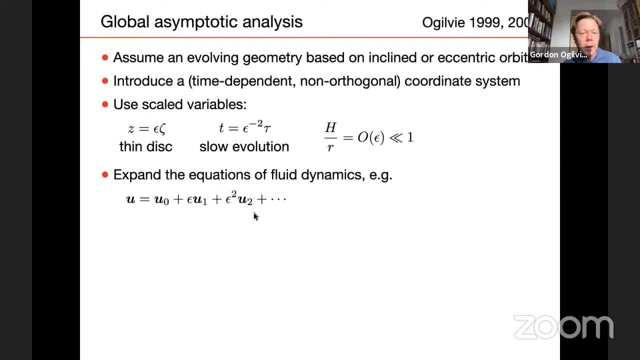 to the orbital speed And, broadly speaking, what you get out of this. at the zeroth order in this expansion you just recover the orbital motion, as you would for test particles. So that's consistent with the assumption of a Keplerian orbit as the leading approximation to the motion. 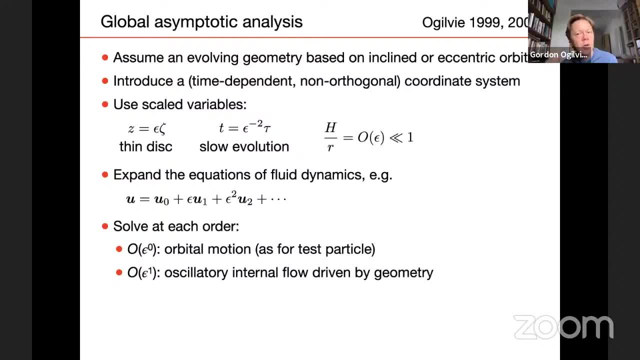 At the next order. in this small parameter we find that there is an oscillatory internal flow within the disk, And this is driven by the geometry of these non-standard disks. I'll say a bit more about that in a moment, And then at the next order. 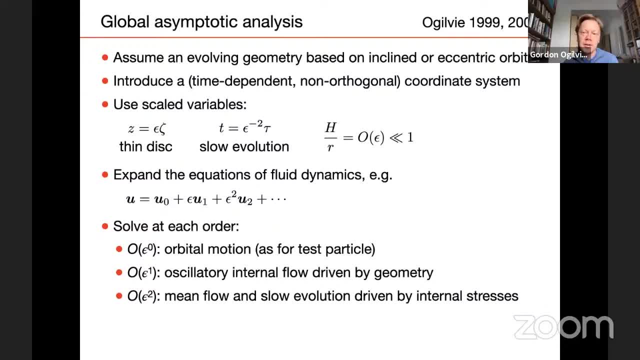 there is a mean flow, which includes the accretion flow that you would have in a standard disk, carrying mass through the disk, causing it to evolve, and indeed a slow evolution of both the shape of the disk and its mass distribution, driven by the various internal stresses And 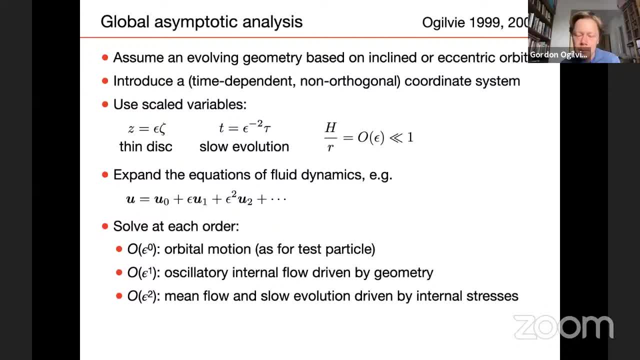 that's ultimately what we're most interested in. So, okay, this is a very mathematical procedure, but it also has a physical meaning. So it's a very mathematical procedure, but it also has a physical meaning, Because this asymptotic analysis, it allows you to separate the different length scales in the 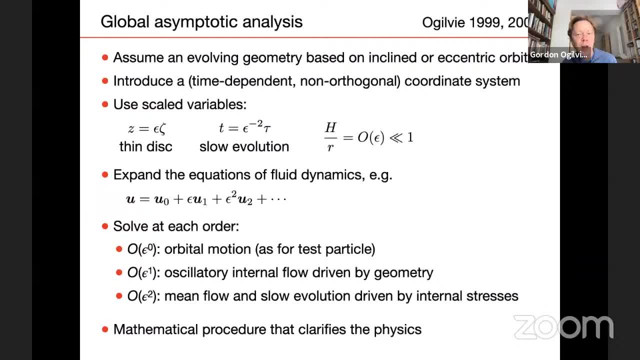 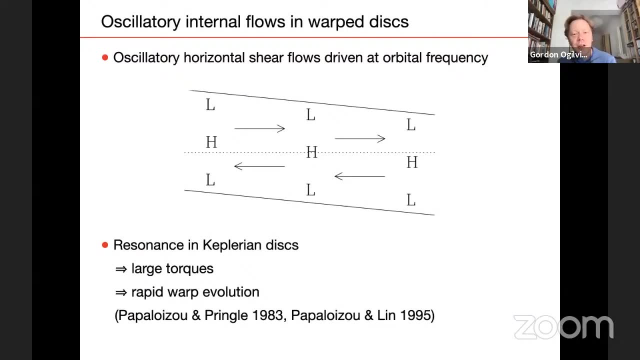 problem and the different time scales and therefore it helps to clarify the physical processes that are going on And it really helps with the interpretation of the physics. So now regarding this oscillatory internal flow that is particularly interesting in the case of warp disks. 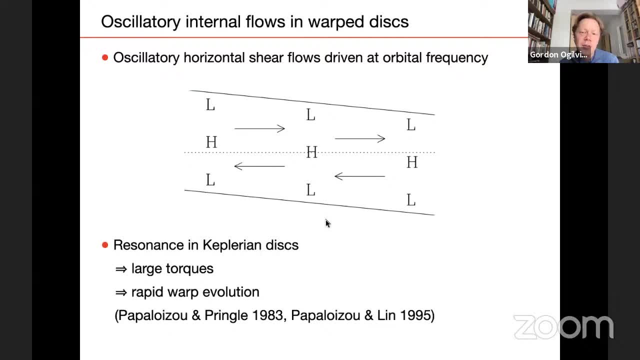 So now regarding this oscillatory internal flow, that is particularly interesting in the case of warp disks. Now, in a standard disk there is a stratification of the pressure in the vertical direction perpendicular to the disk plane. So we have high pressure on the midplane and low pressure. 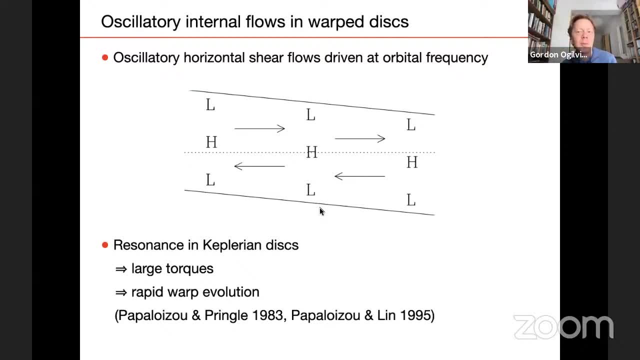 away from it. That's basically a hydrostatic balance between the pressure gradient and, well, the small component of the vertical of the gravity of the central object that's pulling you down towards the midplane. Now, when the disk is warped, that corresponds locally. 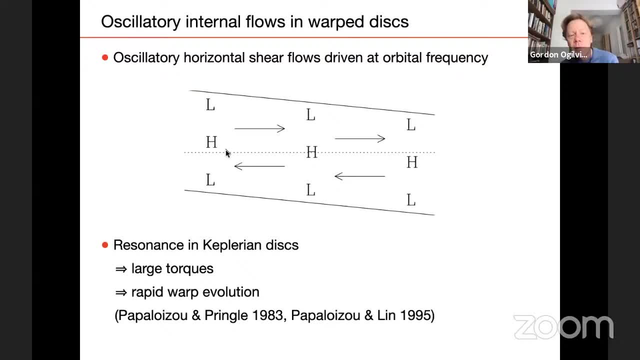 to a misalignment between the midplane of the disk and the local orbital plane And that introduces some horizontal pressure gradients which have this sort of arrangement. This is like a cross-section through the disk And now, from the perspective of the fluid that's. 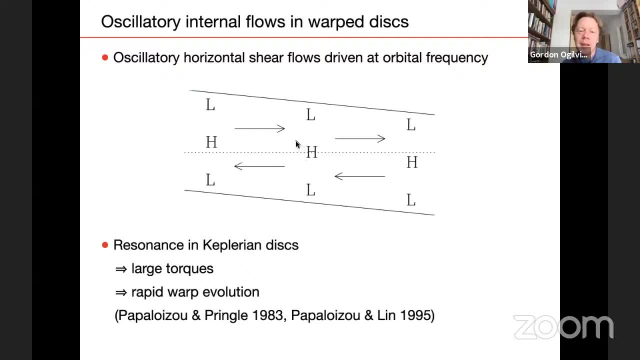 orbiting through this structure. it sees these pressure gradients as a varying at the orbital frequency, which is also the natural frequency of horizontal motions, because the epicyclic frequency, at least if the disk is Keplerian, the epicyclic frequency 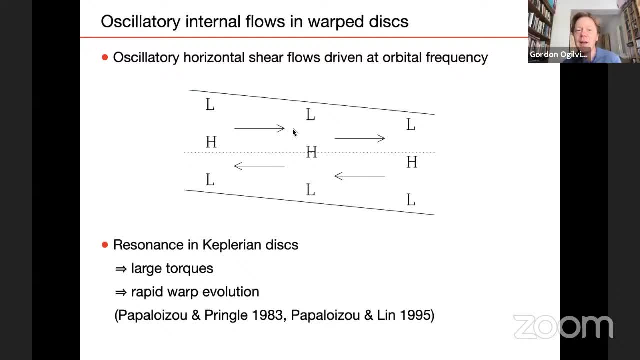 which is the natural frequency of horizontal perturbations of an orbit, is equal to the orbital frequency, And that means that a resonance occurs in Keplerian disks, causing these internal flows to be anomalously rapid and correspondingly there are large internal torques, and that means 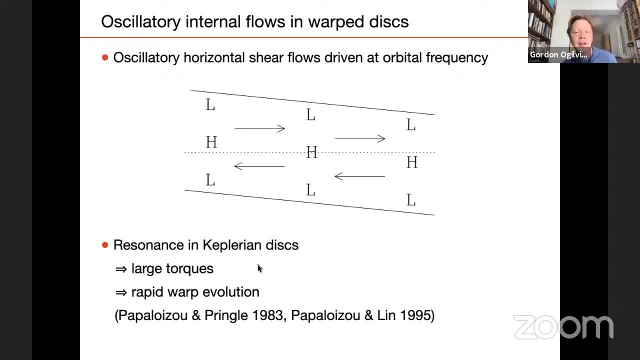 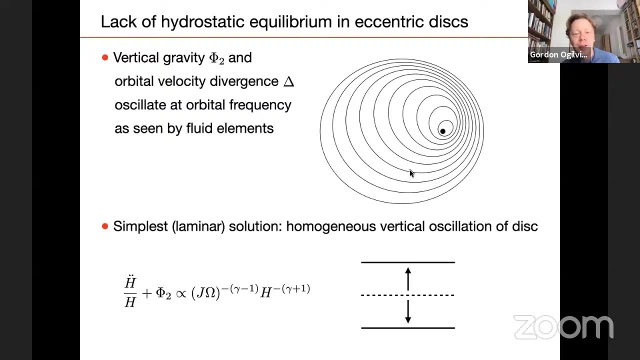 that warps evolve especially rapidly in Keplerian disks, which are of course the most important ones in astrophysical applications. Now, in eccentric disks there's another important phenomenon: that, as the fluid flows around and lipidizes, the orbital velocity field in the plane of the disk has a non-zero divergence that oscillates. 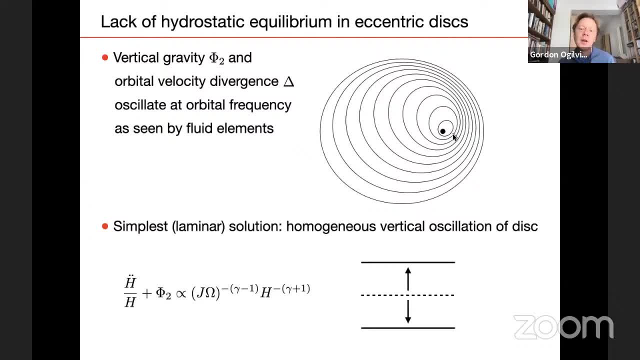 at the orbital frequency as well. So the orbital velocity field in the plane of the disk has a non-zero divergence that oscillates at the orbital frequency as well. So both of these are actually will cause the disk to oscillate vertically. 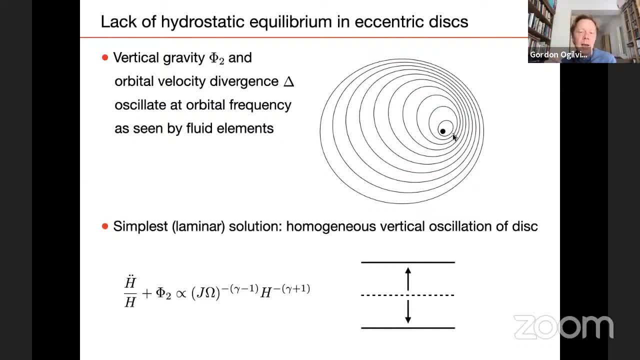 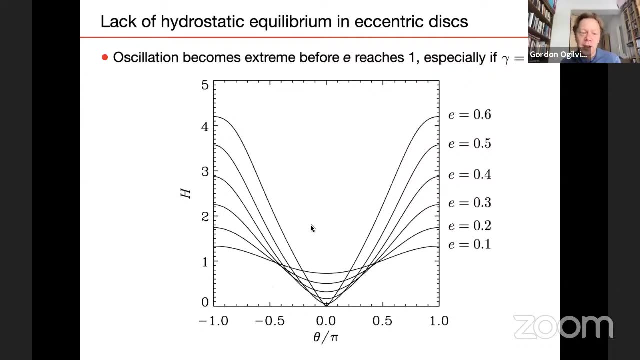 not to be in hydrostatic equilibrium, And so it undergoes a forced breathing oscillation which can easily become non-linear. So here, for example, is a calculation of the variation of the scale. height of the disk with azimuth around. 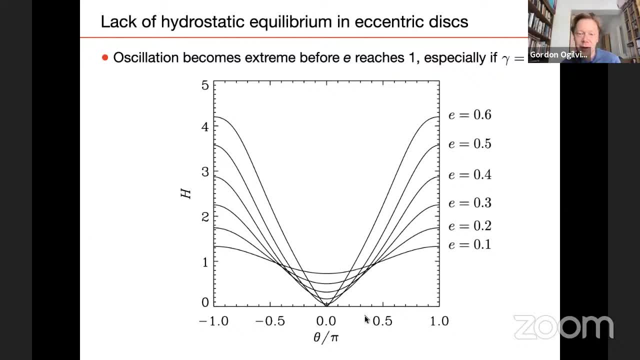 and a disk with a constant eccentricity And we can get into a very extreme vertical oscillation. especially if the disk is isothermal, which means it's very compressible, The scale height can become absurdly small, actually at pericenter, if the eccentricity. 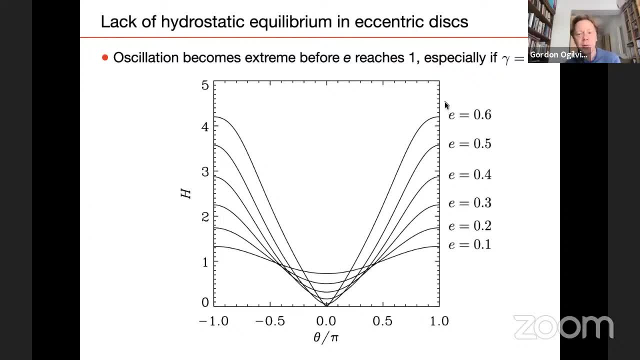 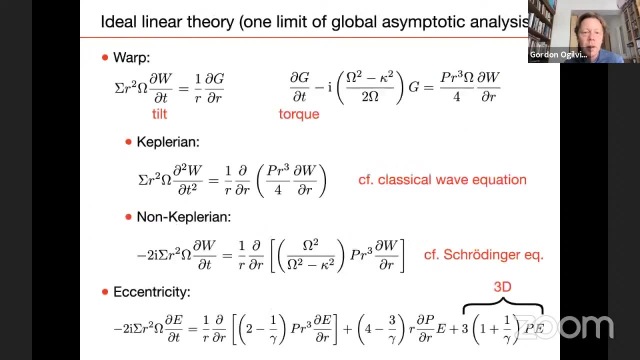 is more than about a half, And this sort of thing turns out to be very important for the tidal disruption of the disk. Now, if you like equations, here are some equations. This is illustrating what some of the equations that can be derived in the case of ideal linear theory. So for an inviscid disk where only 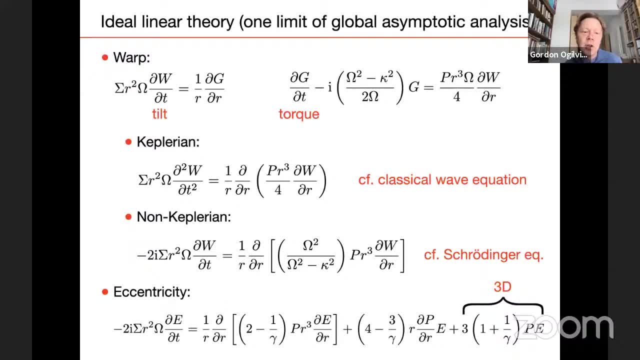 pressure is contributing to the evolution, basically. So warp disks can be described in a linear approximation by a pair of initial equations like this: One for the tilt and another for the internal torque associated with these internal flows, And basically, in the Keplerian case, these combine to produce something like a classical wave equation for the. 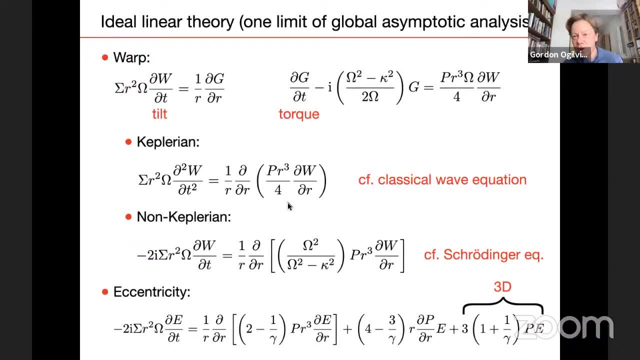 warp, saying that the warp propagates radially through the disk as a result of pressure at a speed that's some fraction of the sound speed in the disk. If you had a significantly non-Keplerian arc, Thanksgiving was just a proper pun for P. 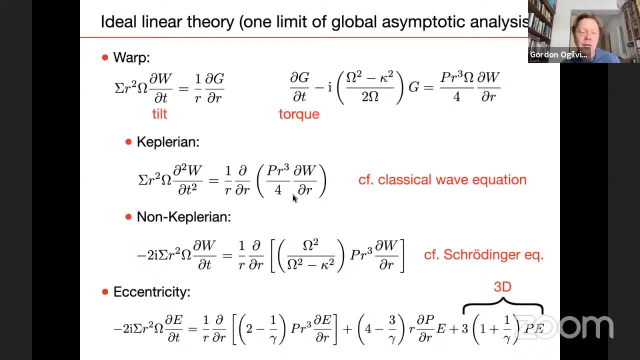 Versus some JE라고 analyzed noise-to-wave specific above here. So course. for example, if you had a height-like concentration of catering and senzaptanca for say관og, enough of a Attack band and an inverse of thedıagonal form, on the other hand, that would destruct matter from aissement. 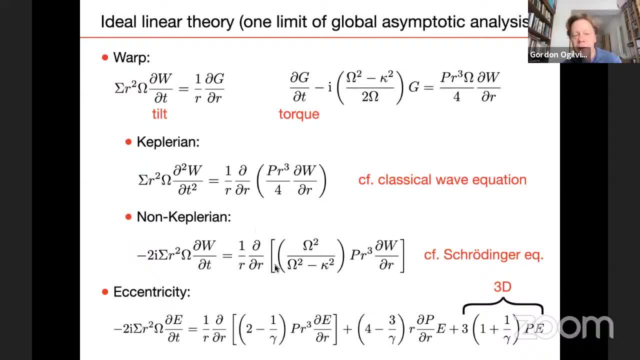 So then, of course, if these inputs come from the Israel root of the Ketchum formula, then all we have to do is determine the total force non-Keplerian disc. then you would get something more like a Schrodinger equation, a dispersive 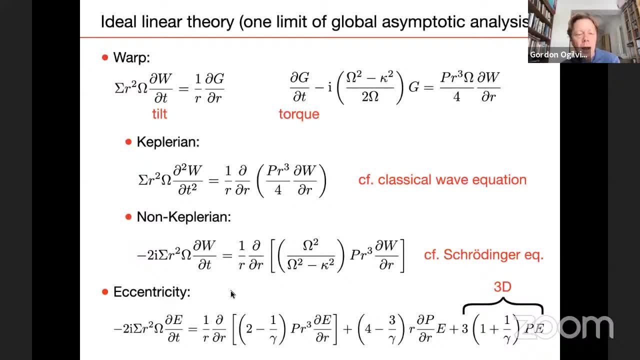 wave equation. And then, in the case of eccentricity, for small eccentricities we do get something similar to a Schrodinger equation, a dispersive wave equation for the complex eccentricity, And there's a distinctive term here due to the 3D effect- this vertical 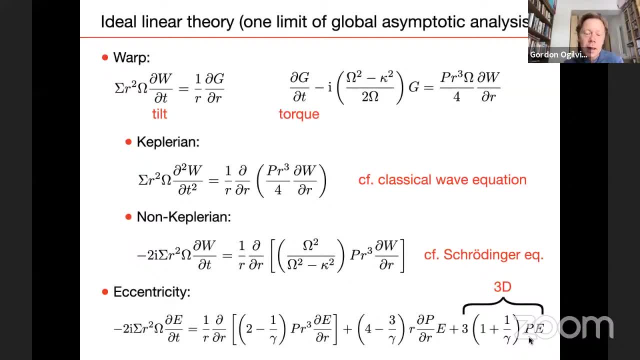 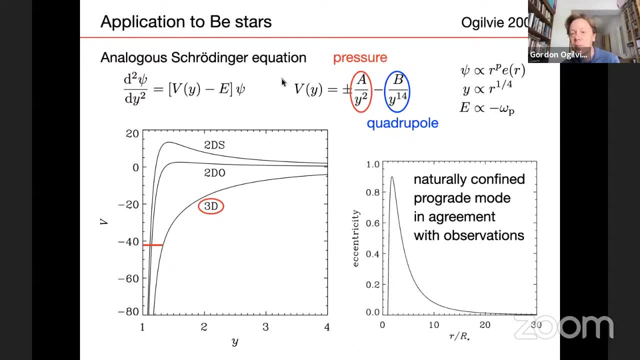 breathing oscillation that I mentioned. So one application of that actually is to the observed eccentric discs around BE stars, these massive and rapidly rotating stars that expel a circumstellar disc. So, as I said, the eccentricity equation can be converted into an analogous Schrodinger equation And the problem 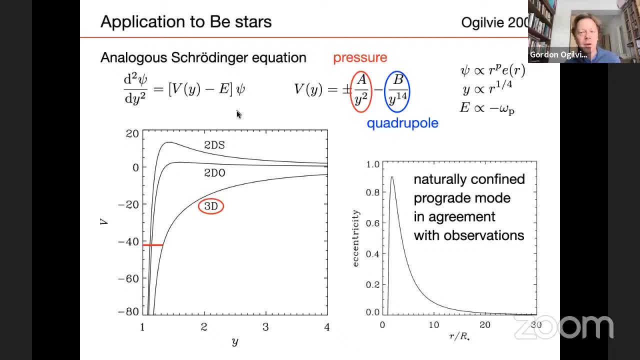 of finding an eccentric mode around a BE star is equivalent to looking for a bound state of the Schrodinger equation in an effective potential. well, And it turns out that this 3D effect that I mentioned, due to the pressure and the vertical oscillations, produces a deep 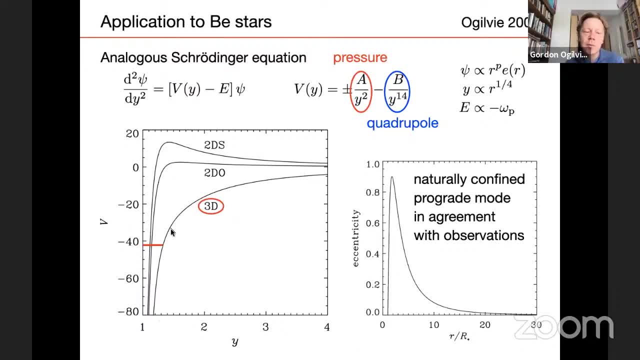 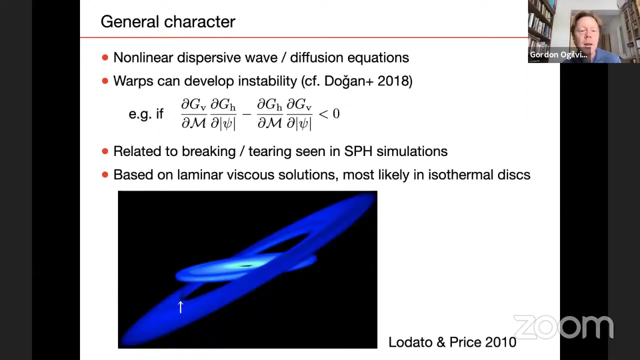 effective potential. well, in these discs. Now, more generally, these evolutionary equations are nonlinear and they can be very diffusive wave equations. They also have a diffusive character if dissipative effects such as viscosity or modeling turbulent stresses really is included, And it has been found that well. 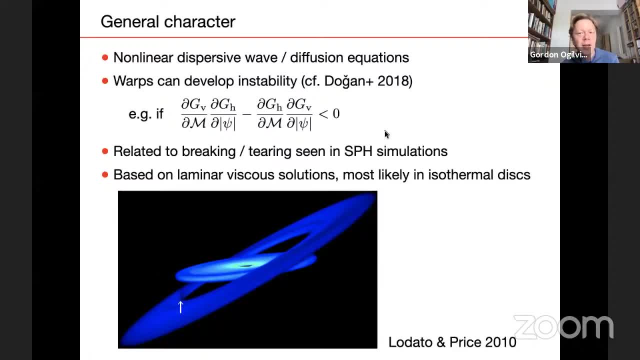 these evolutionary equations can predict instability, sort of diffusive instability. if, for example, the diffusion coefficient for the warp is a decreasing function of the amplitude of the warp, You can get diffusive instabilities in this type of nonlinear diffusion equation And that is thought to be related to the onset of the breaking of these. 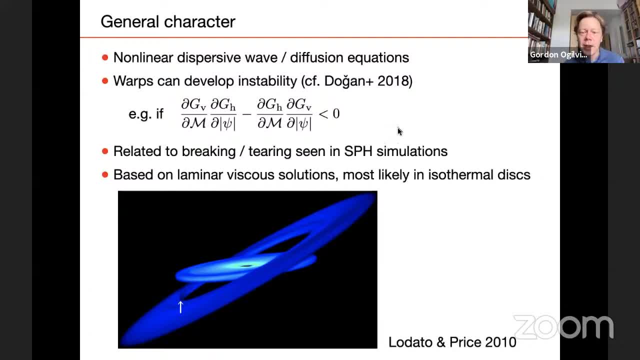 warp discs beyond a critical amplitude, and something that deserves further investigation. I mean, what I would say about that is that this effect is seen in basically laminar viscous flows and also it's most likely to occur in the isothermal discs, which are the ones that 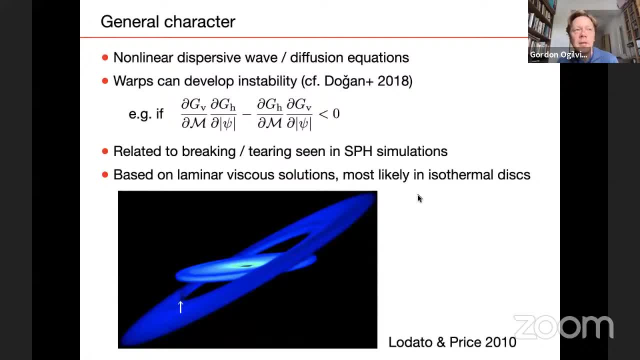 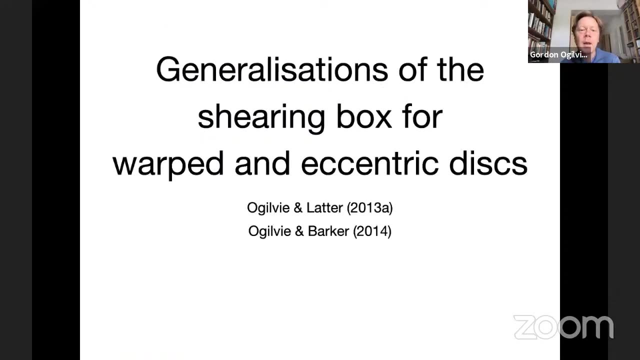 have usually been simulated, because in that case there's no thermal feedback between the presence of the warp and the behavior of the disc. So that poses a limitation, basically, on how much torque it can transfer without breaking. Okay, well, I would like to mention 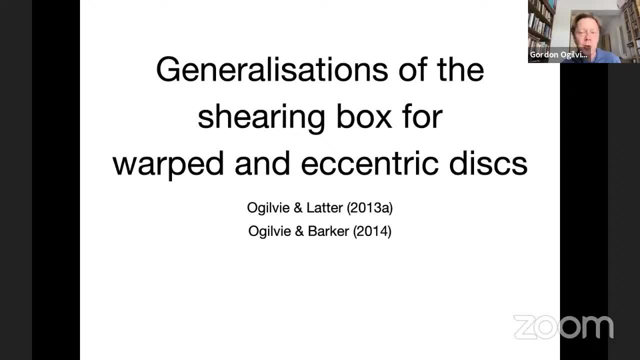 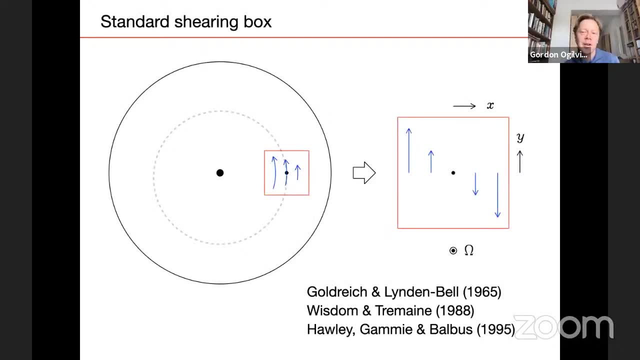 yes, some of the generalizations of the shearing box model that we've worked on for warped and eccentric discs. The standard shearing box is a classic local representation of an astrophysical disc. We just focus in on a patch of the disc and represent it as a uniform shear flow in. 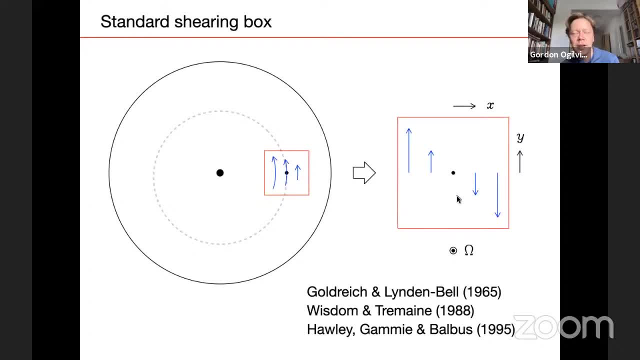 a rotating frame of reference, And this model has been widely used for both analytical and computational studies, And it's been used for a number of other studies, such as the studies of the local physics of discs, waves and instabilities and turbulence, and so on. 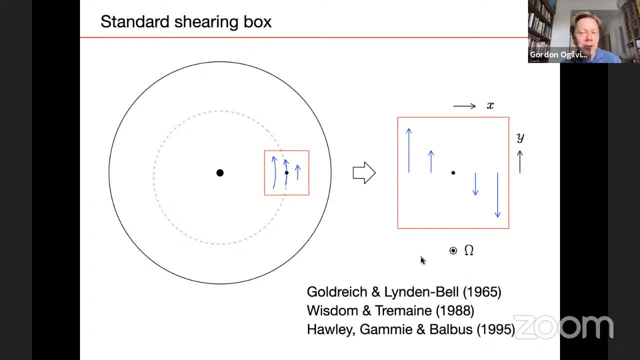 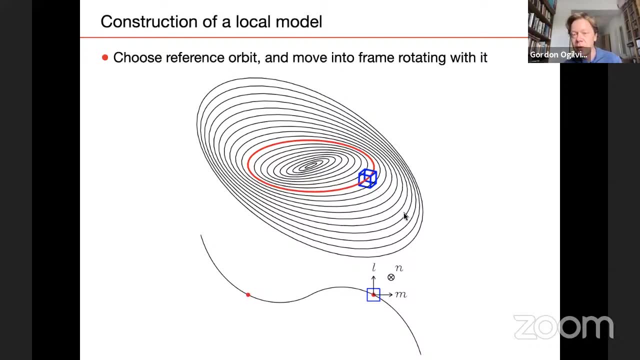 But it is based on a circular coplanar disc. Now for a warped disc we can made of variably inclined circular orbits. we can do a similar construction, That is, pick out a reference orbit somewhere in this disc and go into a rotating frame that rotates with this orbital motion. 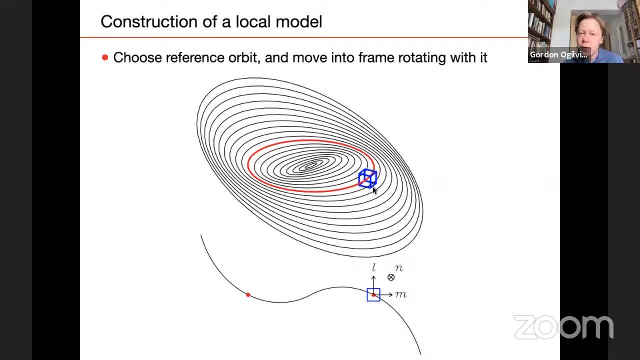 And now, from the perspective of this local frame of reference, the geometry of the disc oscillates at the orbital frequency, at least in as much as the shape of the warped disc is fixed in the inertial frame. So as we go around, this box sees this oscillating geometry, which is 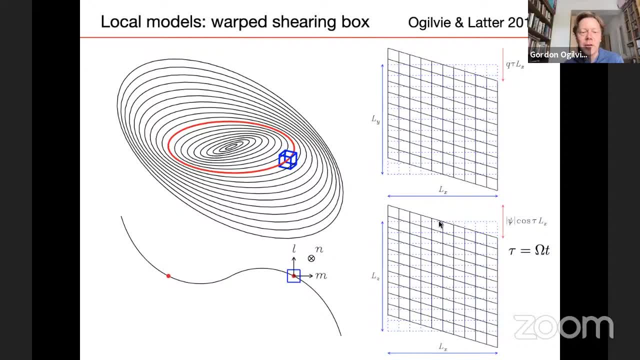 responsible for forcing these internal flows And this can be built into the coordinate system So that we have now an oscillatory vertical shear like this due to the presence of the warp, in addition to the steady orbital shear in the plane of the disc. 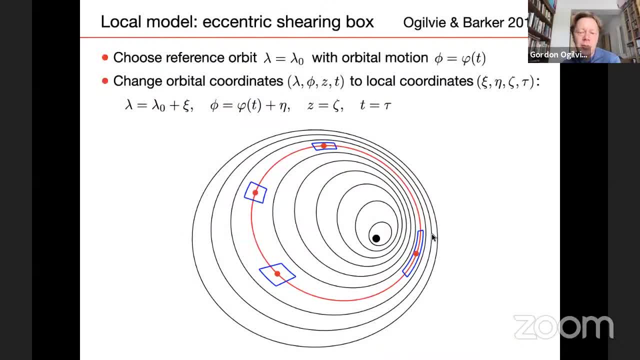 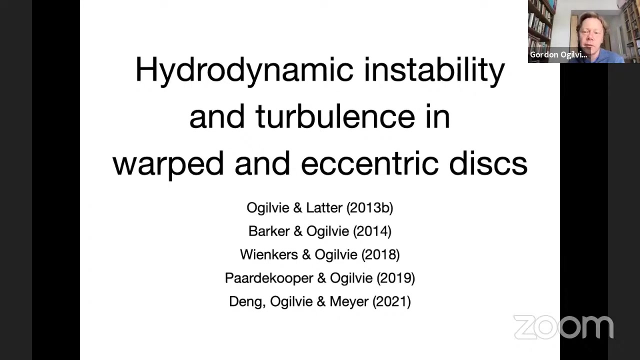 Something related can be done for eccentric discs by making boxes that move and are deformed according to the orbital motion, And in general that involves some oscillatory compression here in the horizontal directions. Okay, And we have used this type of computational model to understand the onset of hydrodynamic. 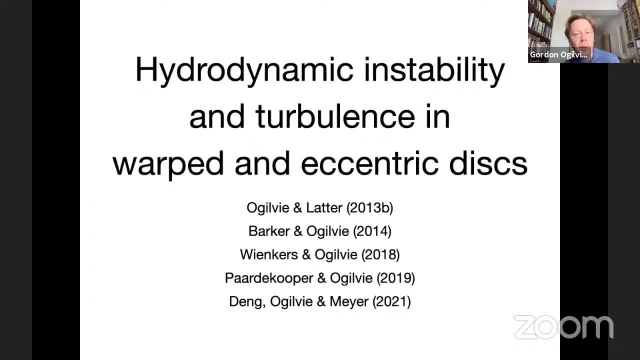 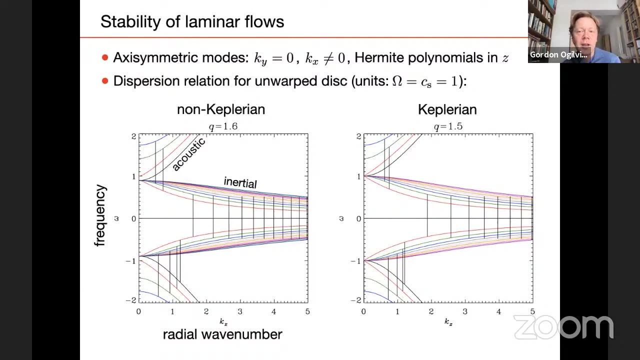 instability and the production of hydrodynamic turbulence in these flows, Which is, it's, a novelty, because people generally have thought that hydrodynamic turbulence doesn't occur in astrophysical discs, that you need magnetic fields to produce turbulence. So I mean, roughly speaking, what's happening here is a parametric instability, a parametric resonance. 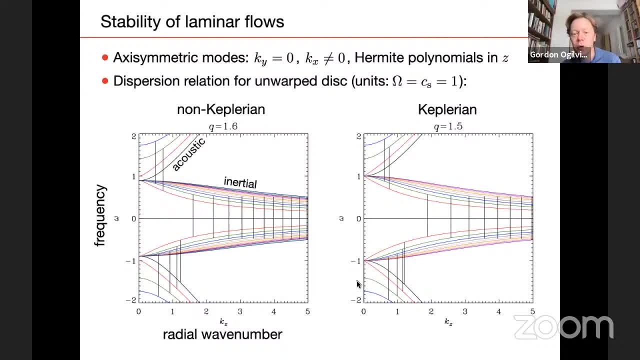 which means that you're taking- and this is the dispersion relation for waves- in a disk. there are high frequency acoustic waves and low frequency inertial waves restored by the Coriolis force. So here we're finding pairs of inertial waves which are you know. 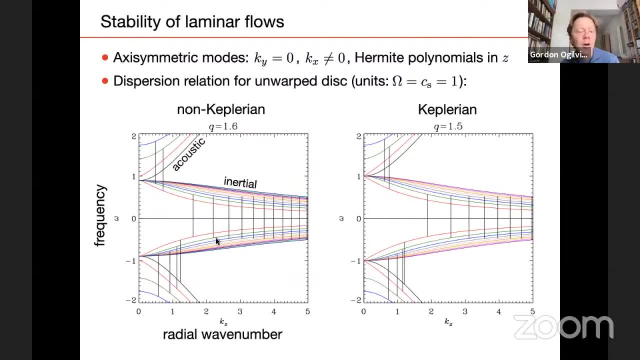 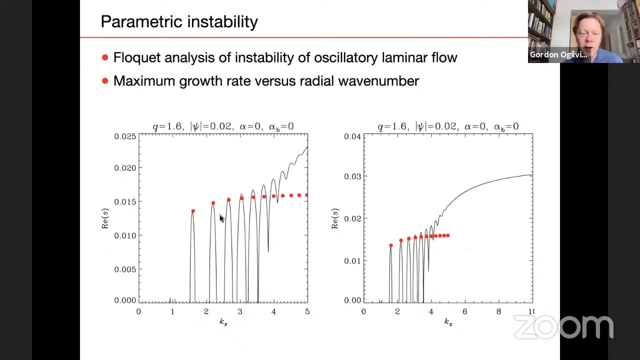 waves whose frequency differs by the orbital frequency and they have the same radial wave number. this pair of waves can be destabilized by coupling to the warp or the oscillatory geometry, And that leads to an instability with a growth rate that can be calculated. 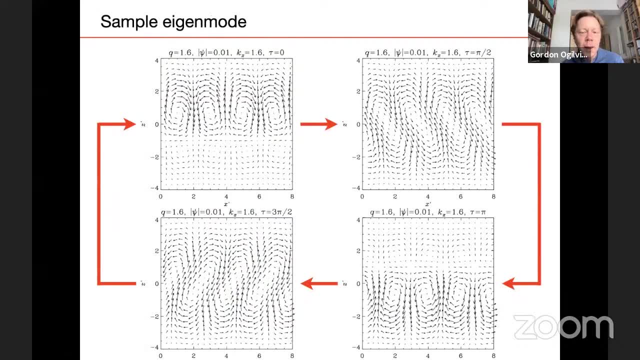 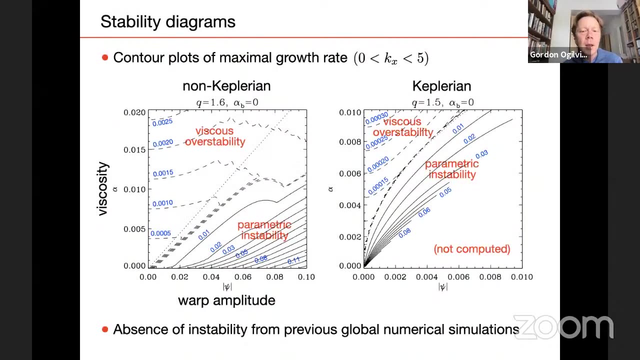 and increases with the warp amplitude. The unstable modes are basically feeding off the oscillatory shear flows in the disks. They produce Reynolds stresses that extract energy from that and grow as a result. And well, at least at the time we were doing this work, there was no evidence of this type of instability in any numerical simulations of 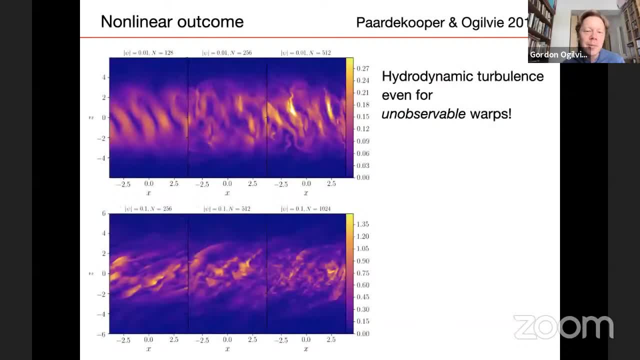 warp disks. So we set out to do some local computations using this warped shear. This is a measuring box model. This is where Simeon Pardekope And so here we showed that the instability leads to hydrodynamic turbulence. Now, interestingly, this can occur even if the warp is extremely. 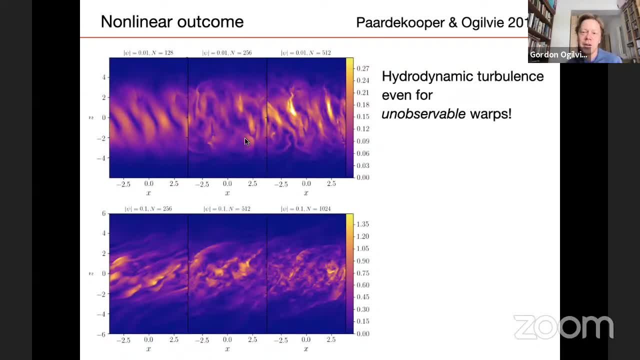 small, And that's because of this resonance in Keplerian disks that the magnitude of the internal shear flows can be very significant, even if the warp is very small, So small that it would be unobservable. So we may have hydrodynamic turbulence in astrophysical disks that don't even appear to be warped. 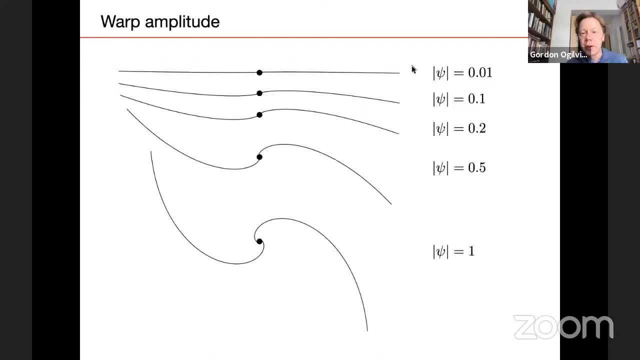 So, for example, at this sort of amplitude where what I call a 1 percent warp- Okay, the nonlinear outcome is often a statistically steady, A hundred percent steady, of course, but this is an entwicpment of thermal dynamics. Now, it's not necessarily quite the same as what we are used to, but these are actually very similar. 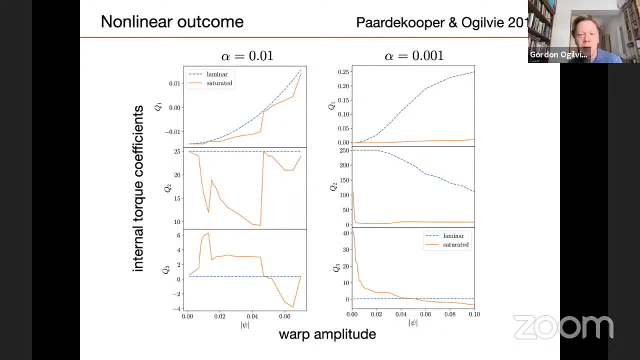 The nonlinear outcome is often a statistically steady, 100 percent steady relationship. So this is one of those approaches that we have applied in these: a hydrodynamic turbulence with measurable properties and it has internal torque coefficients that can be measured And they're different from those of the laminar disk without. 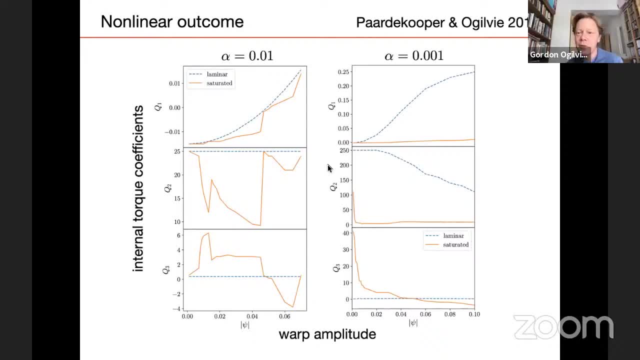 the turbulence And that means that the evolution of the warp and of the disk generally will be different when it enters this turbulent state. But there are some quite complicated issues here to do with hysteresis and the nonlinear nature of the transition to the turbulent state. 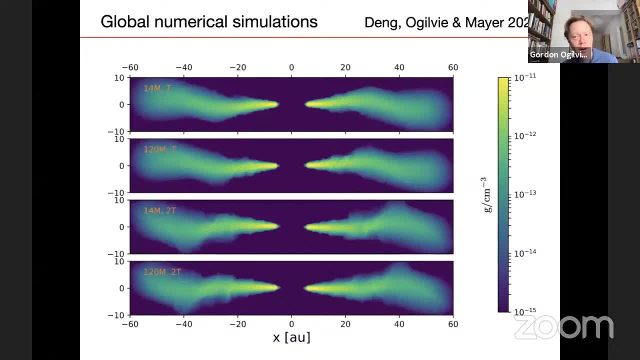 Now, very recently, I've been working with Hung-Ping Deng, who was Lucio's PhD student in Zurich, And he's been doing some very nice global simulations of warp disks, not using the SPH method, but using the meshless finite mass method. 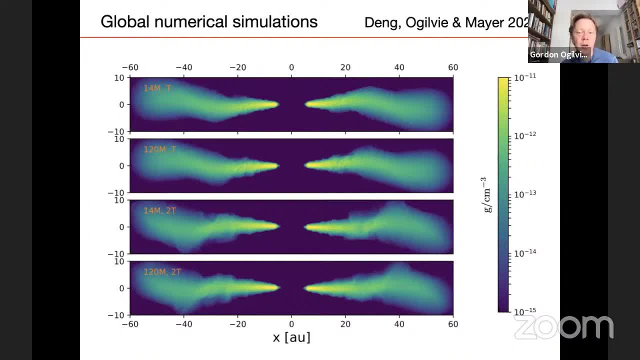 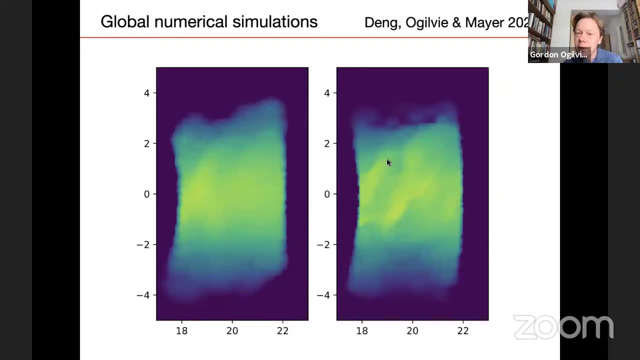 Which has some superior properties. It's better able to resolve these internal flows and small scale instabilities. So using some very high resolution simulations here he was able to find this parametric instability and turbulent motion occurring in global simulations of warp disks. for the first time- The signature of this, by the way- are these sort of oblique. 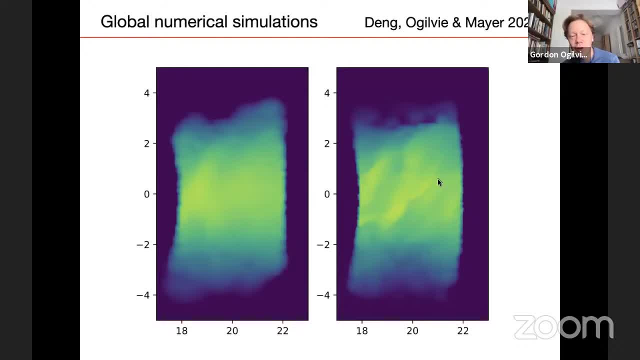 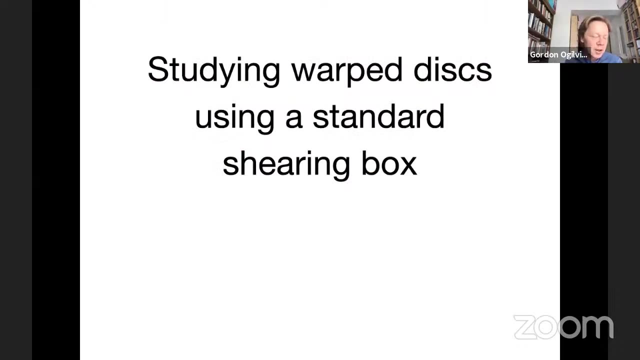 this is showing the breaking nonlinear inertial waves. Internal waves tend to break when they exceed a critical amplitude, And that's what's happening here. Now it's also possible to study some aspects of warp disks actually using a standard shearing box, which means you don't have to recode the 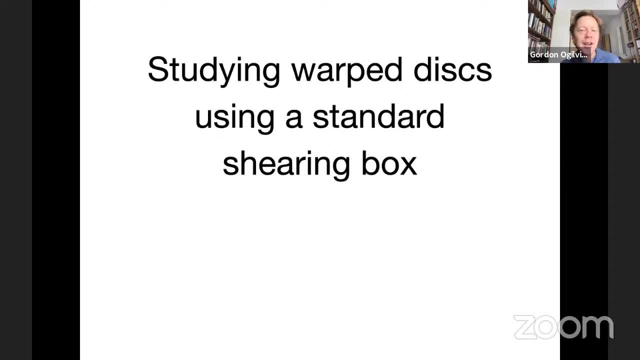 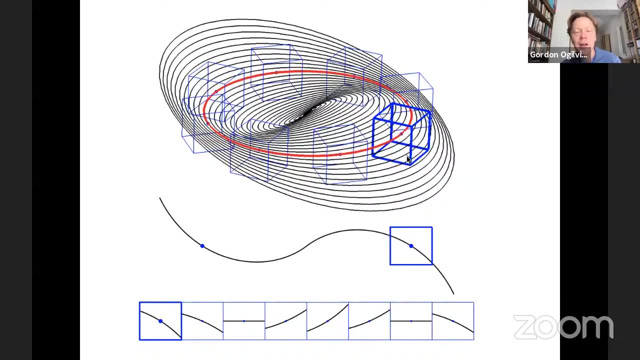 fluid dynamical equations in this funny coordinate system. So that has a number of advantages. So, roughly speaking, the idea is to think of, well, perhaps a larger shearing box. And now, okay, we've got this warp disk. Here I'm sort of plotting the radial. 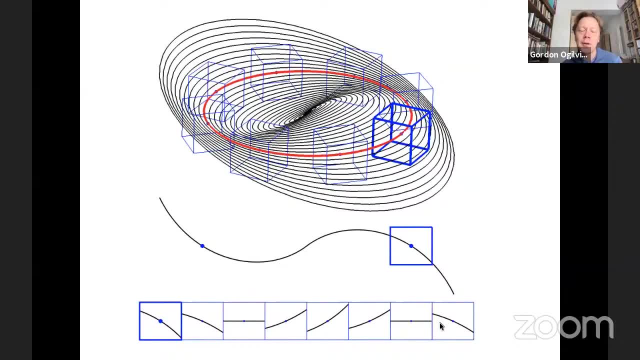 cross-section of a warp disk at various orbital phases, as this box goes around the reference orbit. Now, to the extent that the warp is stationary in the inertial frame. the warp disk is not stationary in the inertial frame. What's happening in this local frame is just that each piece of the disk is. 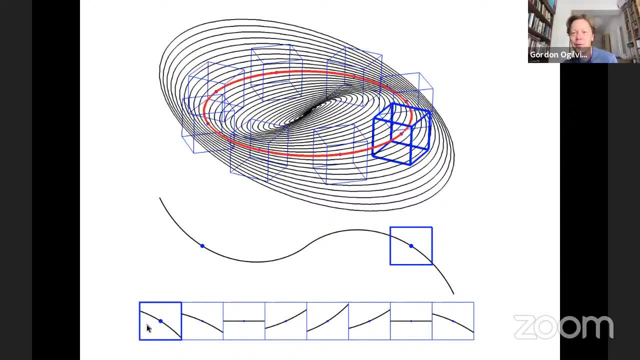 oscillating up and down at the orbital frequency, which is a free motion of test particles. Any evolution of the warp on a longer timescale would correspond to a modulation of this vertical oscillation. So that's what we should be trying to detect. So as a proof of concept, here's a. 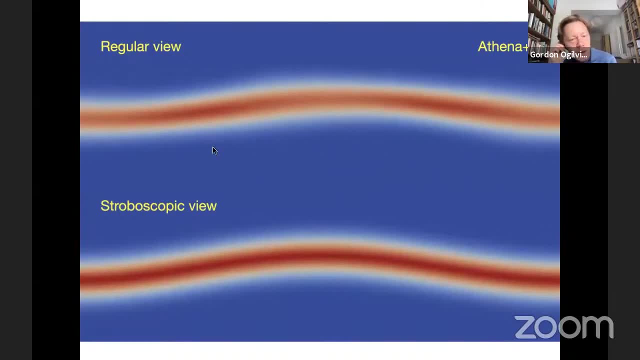 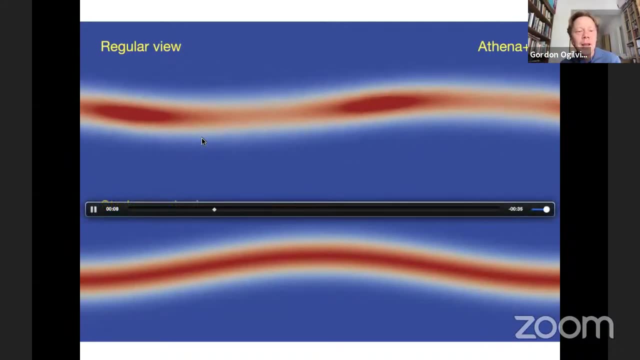 simulation of a very simple setup of a gas disk with this sort of corrugation representing a warp, And okay, you basically see each fluid element oscillating up and down at the orbital frequency. But of more interest is what happens on a longer timescale of many orbits, And we'll see that after. 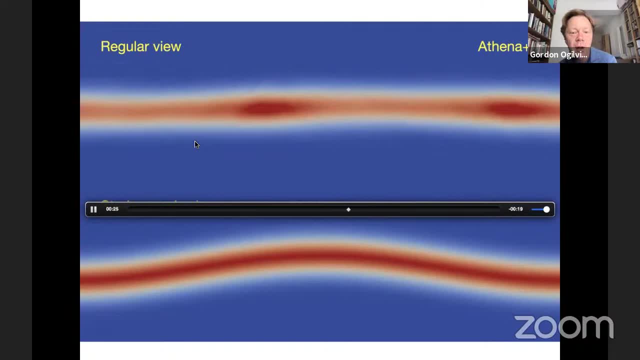 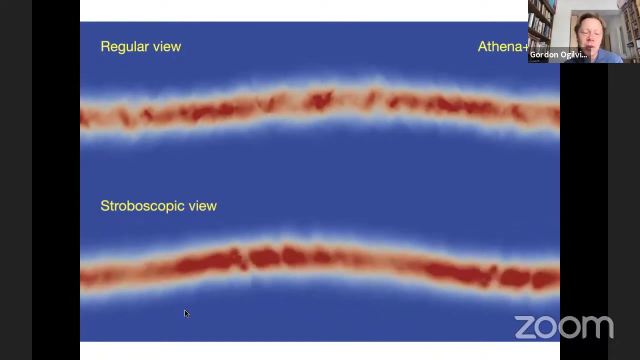 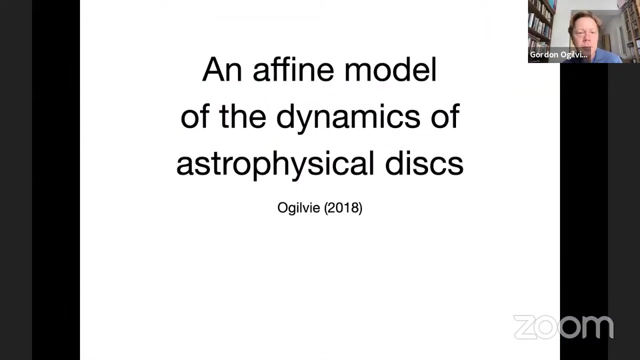 some time, instability occurs. In this case, the parameters are right for this parametric instability. So what I always then do is: I, you y plane the ِّ. it's damped out by the turbulence that results from this instability. Finally, I just wanted to mention this affine model that I worked out, which I think has 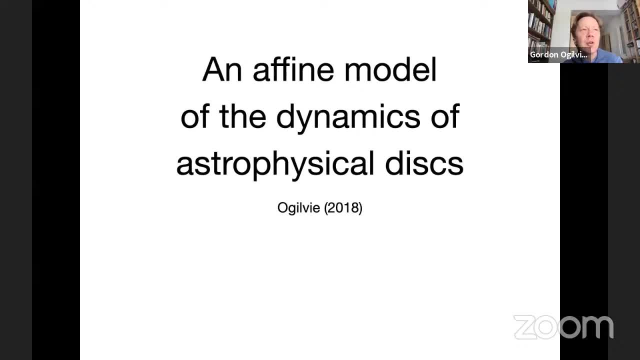 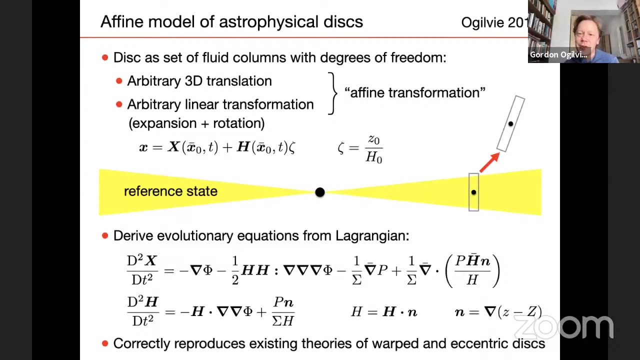 potential to address some of these situations. It doesn't address the small-scale instability, but it could be useful for long-term simulations in which that doesn't occur. This is motivated by the fact that for decades, people have used two-dimensional fluid equations to represent thin disks. That is ignoring completely the vertical. 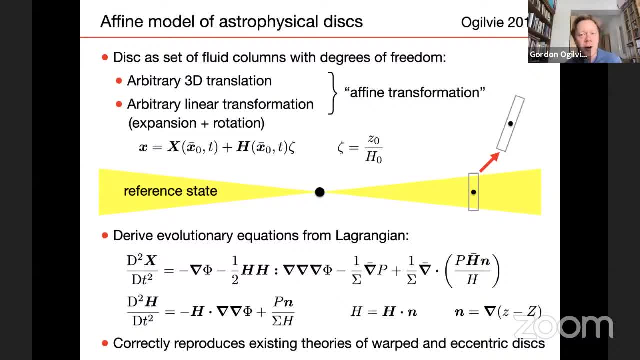 dimension perpendicular to the disk plane. That's actually very difficult to justify. The idea here is to restore certain degrees of freedom. Rather than thinking of the disk as made of fluid elements that can only move in a plane, we think of them as fluid columns that have some vertical extension. 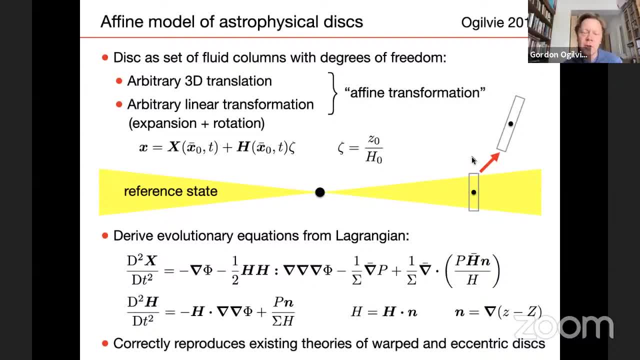 Their translations can take them out of the disk plane, to describe situations like a warp disk. They can also undergo expansions and contractions parallel to their length and they can undergo rotations or tilts, because that is exactly the sort of shearing motion that's happening in some 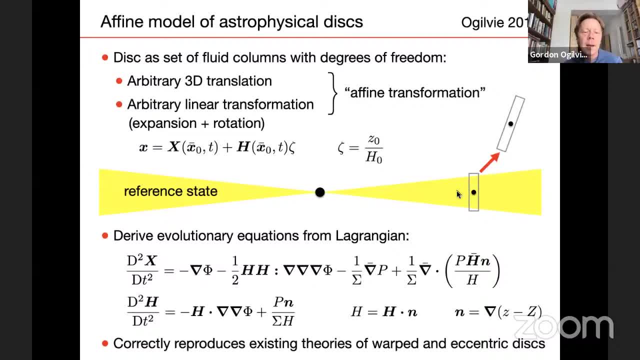 of these systems, Meaning, for instance, the space is so big that if you jump into the disk, the same sort of load increases and the same the mass here would be. But that's the way this whole dynamic work works. So now we've got a lot of possibilities for standing on the earth. This is a clear graph of the Lagrangian equation that we just saw, and it's a really great example of what we can do to say that it's not just glass aproximations, but it's also the way that we can describe the large scale properties of these systems. 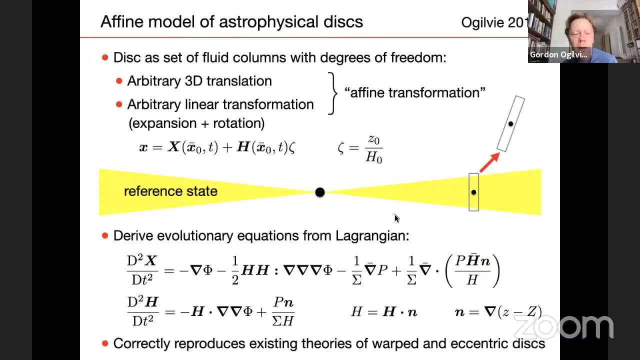 So this turns out to have just the right degrees of freedom to describe the large scale properties of these systems, which then inherits the right sort of conservation properties. So far that's only been done for ideal fluids, but it does, promisingly, reproduce basically everything we know. 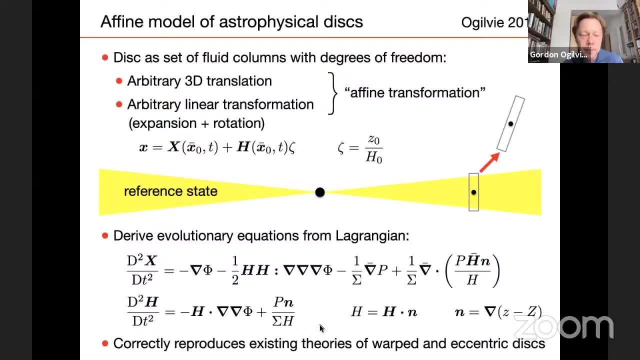 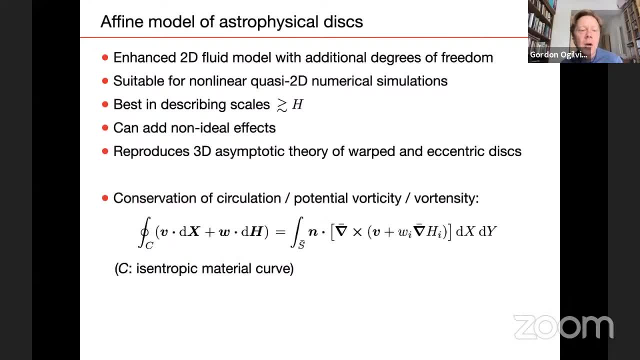 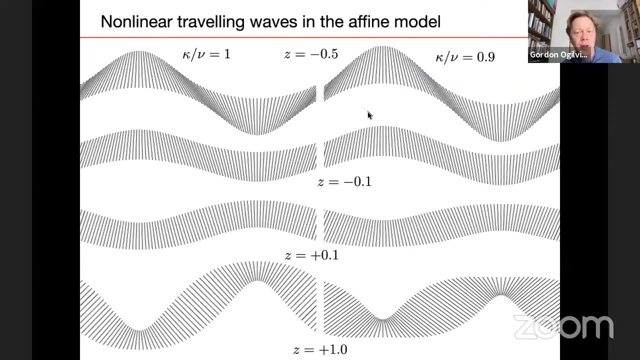 so far about warped and eccentric disks. in terms of the global asymptotic theories. Okay, and just an example of what that can produce When that's combined with the local model. we can, for example, compute nonlinear traveling bending waves, which is a way of understanding the physics of warp propagation. 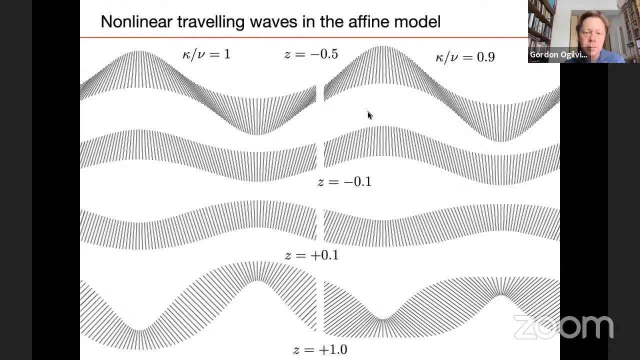 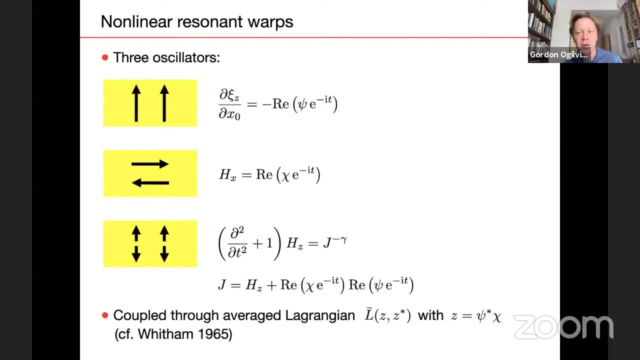 in a nonlinear regime, And one thing that's led to really is a clarification of what the essential nonlinearity in that problem is. It turns out to involve the coupling of these three oscillators: The vertical oscillators, in which the entire disk is just going up and down. 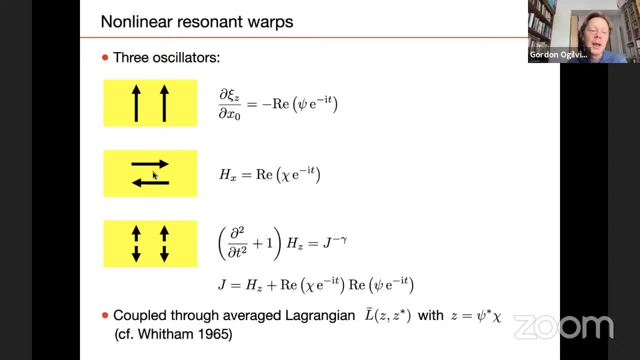 That corresponds to the inclination of the orbits. There's this horizontal shearing oscillator, which is the internal flow excited by the oscillatory geometry in the warped disk, And then this breathing motion, which is coupled nonlinearly in the case of warped disks. 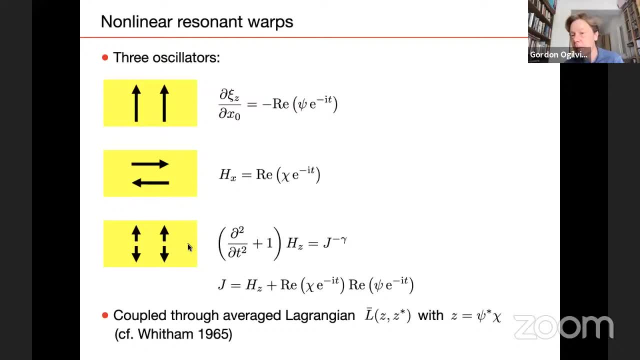 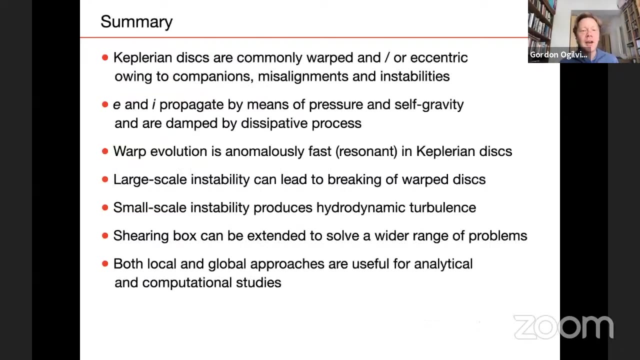 And it turns out to be the nonlinear coupling between these three oscillators. that's the key to understanding the nonlinearity And indeed that we believe is related to the breaking process for the warped disks. Okay, so I see that my time is essentially up. 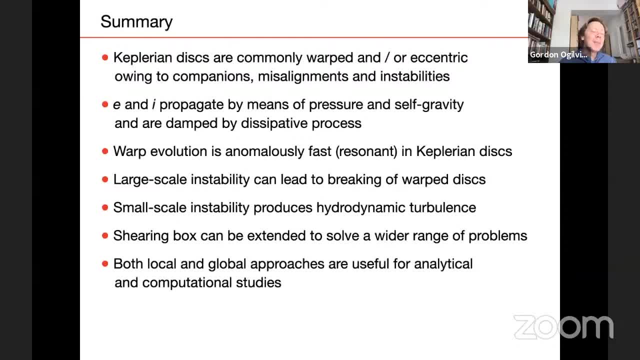 So just to summarize, Keplerian disks are commonly warped or eccentric as a result of companions, misalignments and instabilities. Eccentricity and inclination propagate through the disk by means of pressure and self-gravity, and they're damped by various dissipative processes. 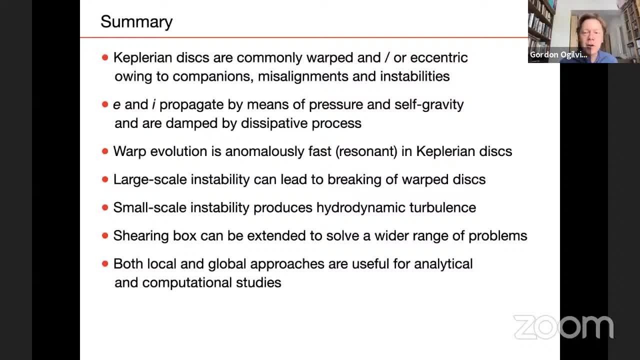 We've seen that warps evolve especially rapidly in Keplerian disks because of this important resonance. There are a couple of instability processes that deserve further study: A large-scale instability that leads to the breaking of warped disks, and a small-scale instability that produces turbulent motion. 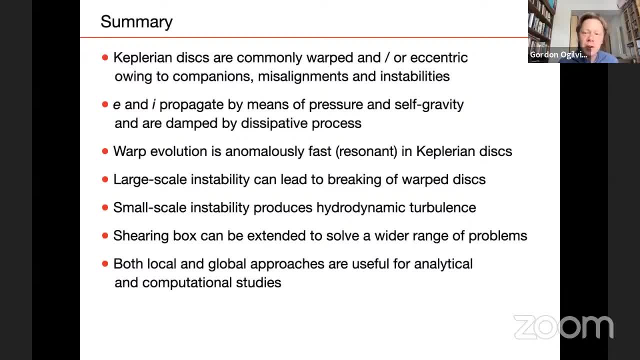 And from the theoretical and computational point of view we've seen that local models can be very effective. The Shearing-Box model can be generalized to study these situations and that's useful for focusing on the small-scale physics. So I'll stop there and I'm happy to take any questions. 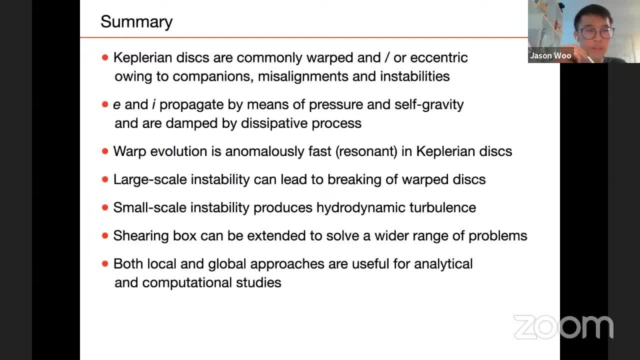 Yeah, so thank you, Gordon. thank you very much for Gordon for giving us a very interesting talk. Thank you, Gordon, for giving us a very interesting talk. Thank you, Gordon, for giving us a very interesting talk. So now we'll move on to the question sections. 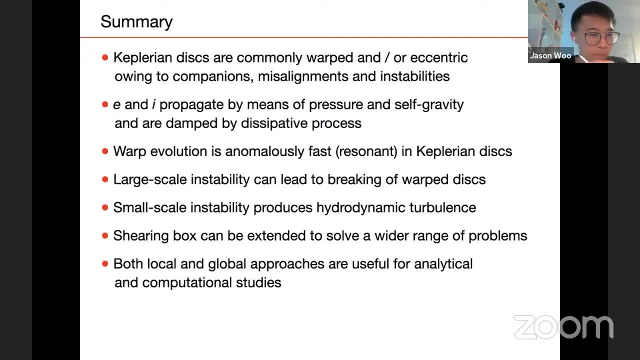 If you have any questions, you can feel free to raise your hand or comment on chat. So I already see a couple of hands here. So we have Andrea to ask the first question, Andrea please. Yeah, thanks for the nice talk. 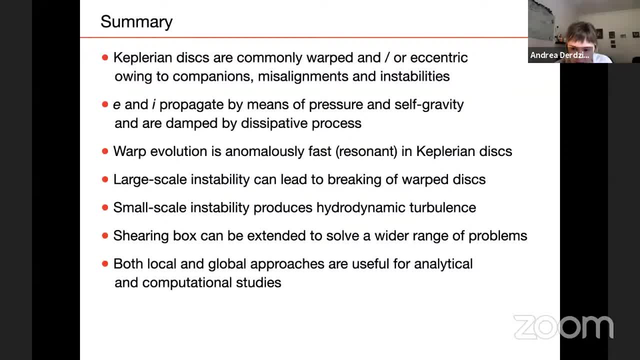 I just have a quick question about the hydrodynamic instability, I guess. I'm wondering if your disk is ionized so it also experiences magnetorotational instability? do you expect these two sources of turbulence to amplify each other, or is there some sort? 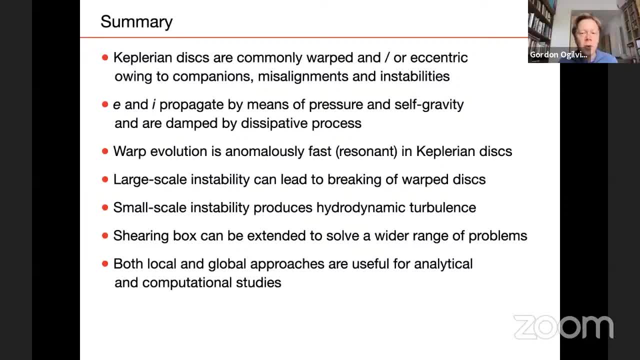 of regulation that could happen. That's a very interesting question And I think, yeah, the competition and interplay between these two quite different instabilities would be very interesting to look at. It may be that, Let's say, if the, If the eccentricity or inclination is sufficiently small, then the MRI dominates. 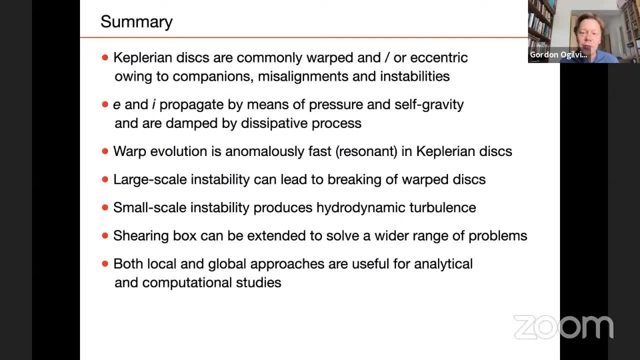 But in other situations the hydrodynamics takes over. It's a little hard to anticipate how they might interact, but I do think that's a very interesting problem to look at. Thank you, Lucio. you can ask questions, Yeah. 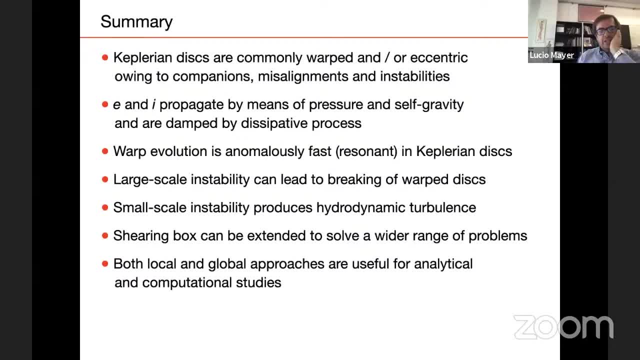 So thanks for the great talk. first, I was very interested in your last part on the affine model. I was wondering: do you think it's possible, with some further work of course, to include in some form the effect of cell gravity? describe the effect of cell gravity actually in your 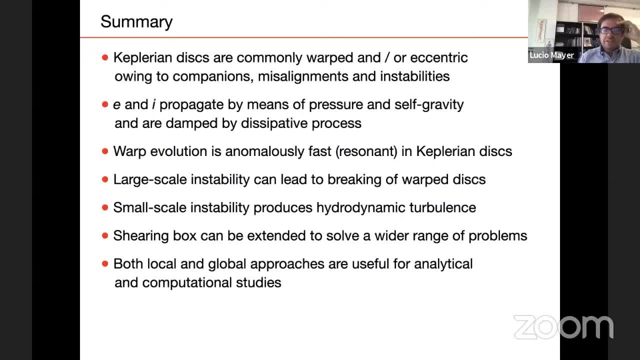 affine model. Because even in the case of the cell gravitating disks, I think a major limitation in our understanding has always been that you do the linear perturbation. Yeah, So in theory, assuming again a thin disk, and so you don't have any three-dimensional. 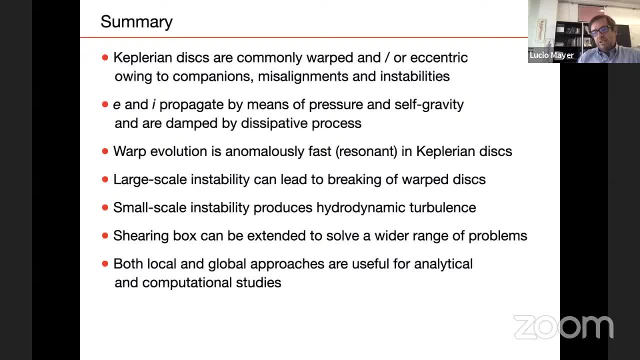 structure there. And then the next step is you do numerical simulations to do the full 3D disk in the nonlinear stage, But there's nothing, There's no approach in between. that would be helpful actually to understand better the transition to the nonlinear regime in a three-dimensional disk. 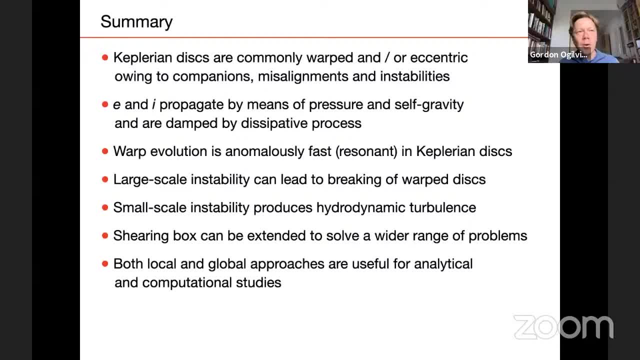 Yes, So that's again a very interesting question And I have become quite interested recently In, yeah, the three-dimensionality of the gravitational instability for another application. But I'm currently working with a PhD student, Callum Fairbairn, who's working on. well, let's. 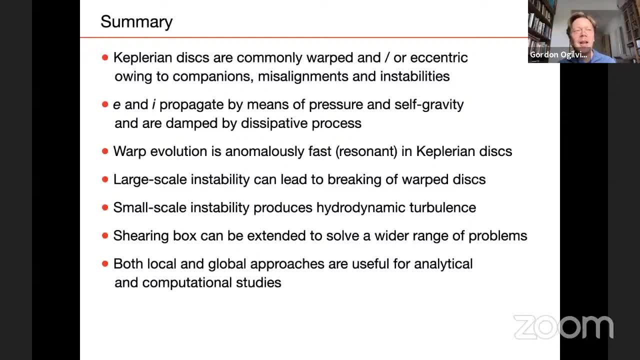 say, a particular version of this affine model, And he has made good progress on incorporating self-gravity into that version. So it's not, Let's say it's not ready yet. Yeah, So I think, although it's not possible to do it in an exact way, I mean it does involve. 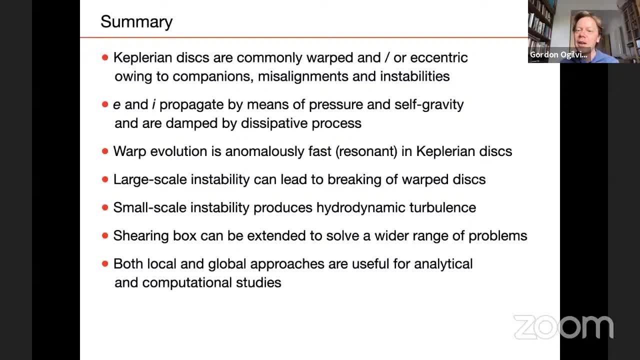 a somewhat ad hoc approximation, but I think with some modeling there is a reasonable way to do this, And the fact that the equations of motion can be derived from a Lagrangian basically means that you just need to model the self-gravitational energy term. 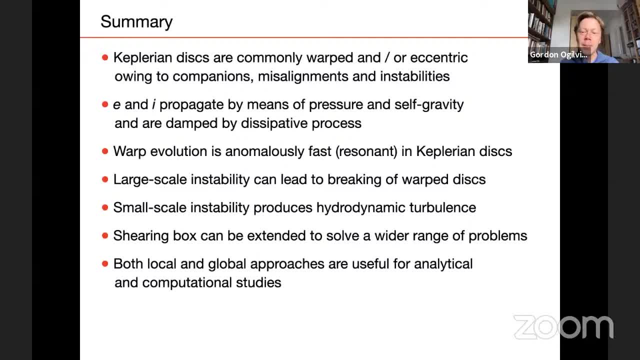 And then everything else follows from there. Oh, that's very interesting. Yeah, Looking forward. So, Jerome, do you want to ask a question? Yep, Hi, Gordon, Very nice talk. Thank you, Rima, That was great. 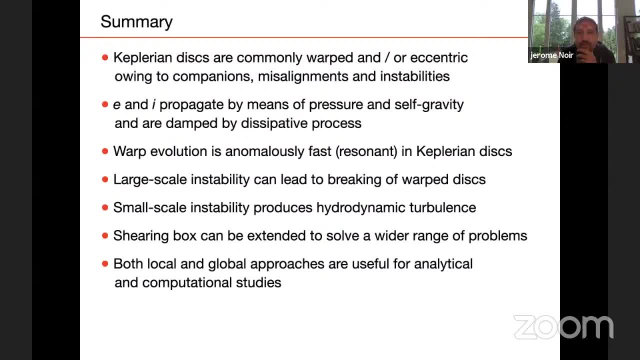 I have a question regarding the possibility to estimate the energy or the power dissipated by this instability using three-dimensional data. Okay, And then the question is: how do you think you can use the model, somehow the work that you've done with Barker, to ultimately get to an observable that could allow to test? 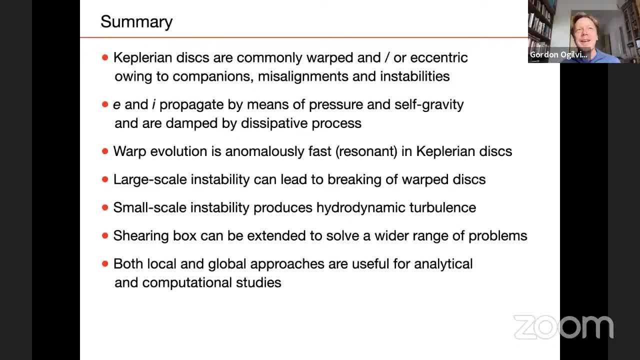 those model? Yes, Well, I haven't thought that far, I have to admit, But I suppose then you would want to. I would be referring to the enhanced luminosity, perhaps, of a rock or eccentric disk as a result of this instability. 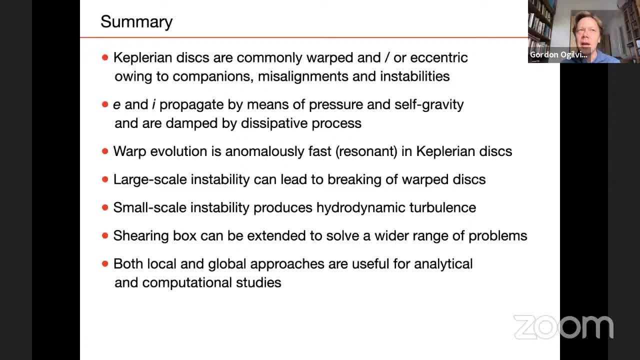 I think that's an intriguing possibility And as we develop models with better thermal physics- because, frankly, the thermal physics content of these models has been quite primitive so far. I mean, it's not like we're dealing with isothermal or adiabatic fluids. 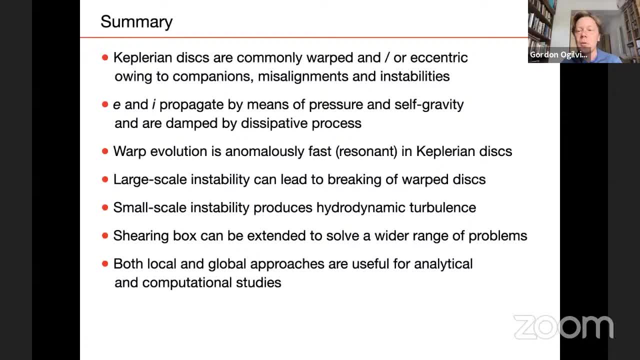 But when the viscous dissipation or turbulent dissipation and radiative cooling are taken into account, that allows the possibility to predict, let's say, the non-axi-symmetric emission from these situations, which has some possible observational consequences. But maybe you were thinking of a more theoretical. 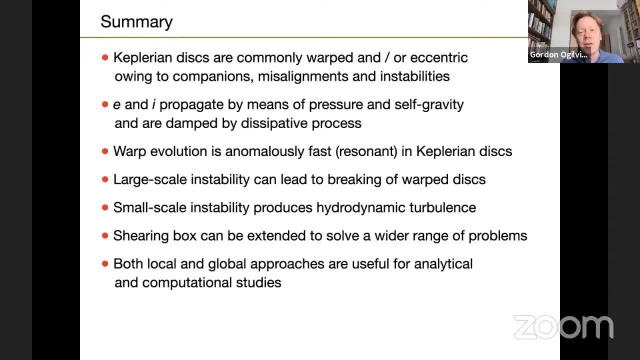 way to estimate this energy dissipation. Thank you, So next Will Herr. Do you want to ask a question? Yeah, Thank you, Gordon, very much for this wonderful talk. I have a question concerning this generation of turbulence. I mean, it seems to me that when the simulations were continuing, that the warps disappear. 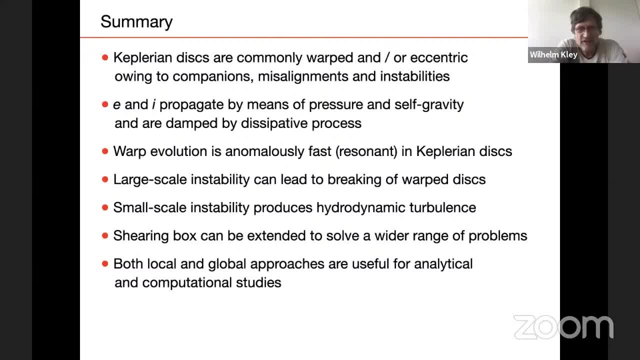 slowly. So doesn't the turbulence warp then against the initial state that you have? Or how is the long-term evolution of that process? Well, that's a very good point. And, of course, if you just had a free, a freely decaying warp, then the fact that the 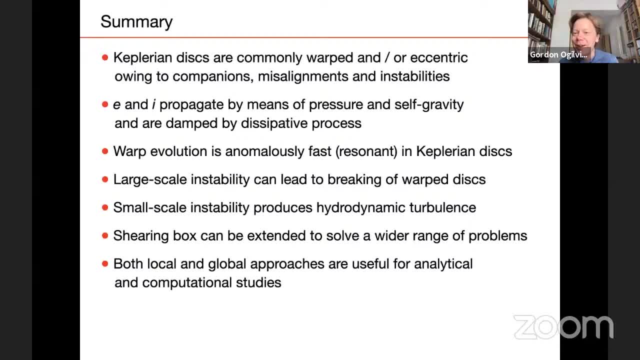 warp produces turbulence that accelerates the decay of the warp would indeed tend to produce a self-defeating process here. So I guess we would have to rely here on the idea that the warp is forced by some misalignment in the system, which cannot go away on a short timescale.